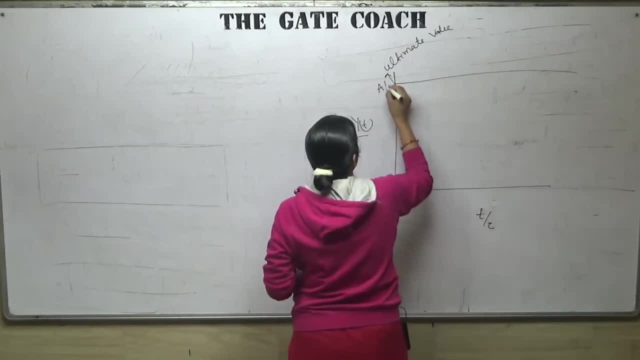 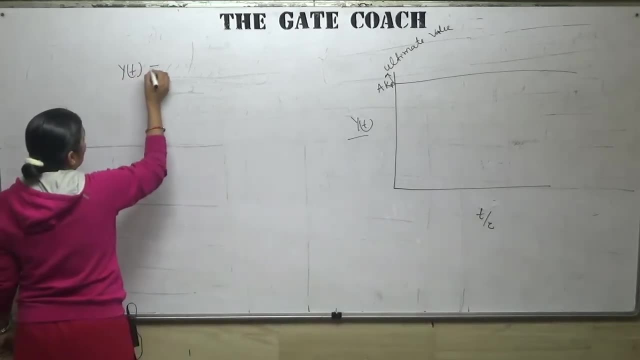 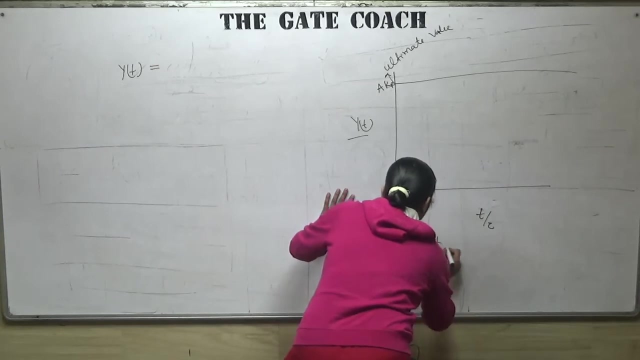 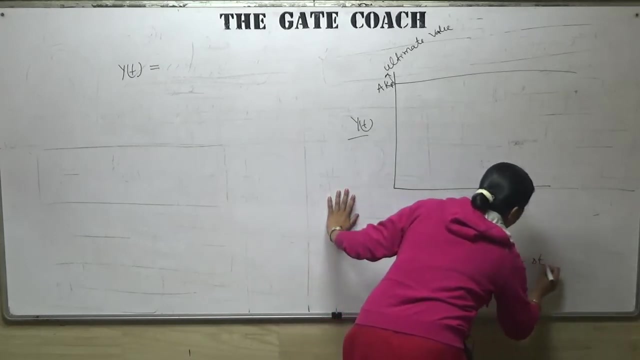 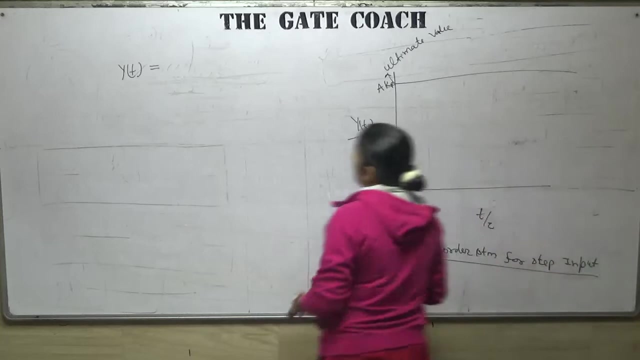 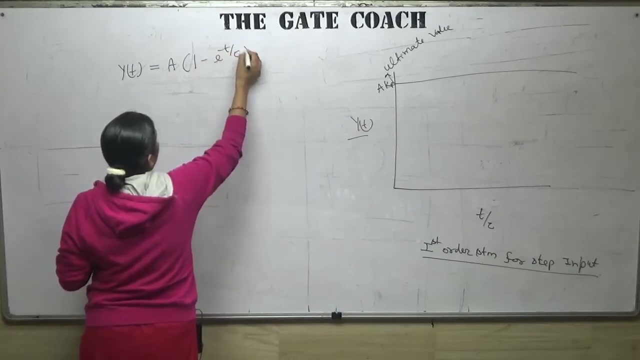 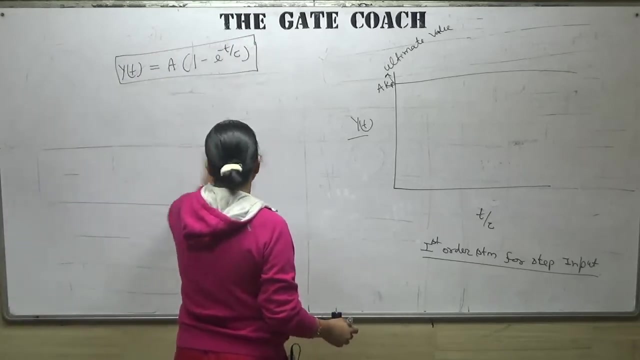 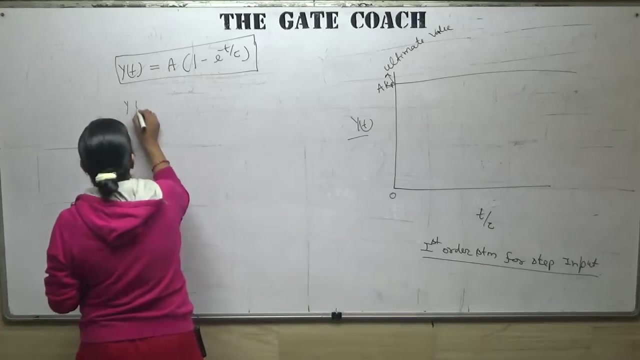 Right, So your equation, the response equation, yt. that comes for the step input. This graph is for the step input, First order system for step input, First order system for step input. Right? So the equation, the output response equation that we will get is a into 1 minus e to the power minus t upon tau. So this is the equation. So from this at time, t is equals to 0. What is the value of this? from by t, t is equals to 0, e to the power minus 0, 1 minus 1, 0. Right. 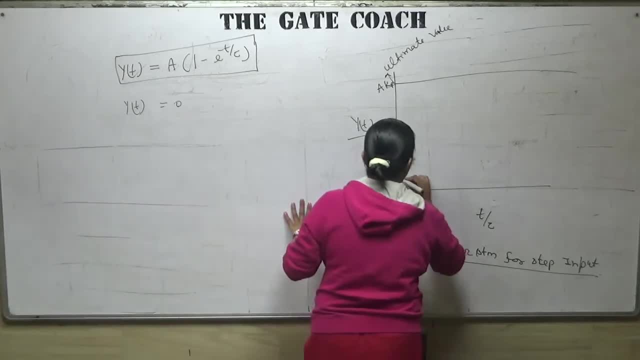 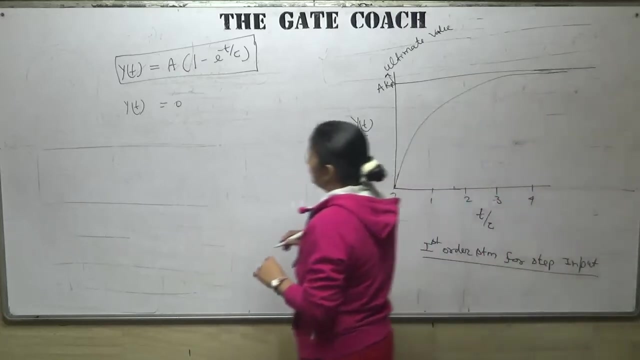 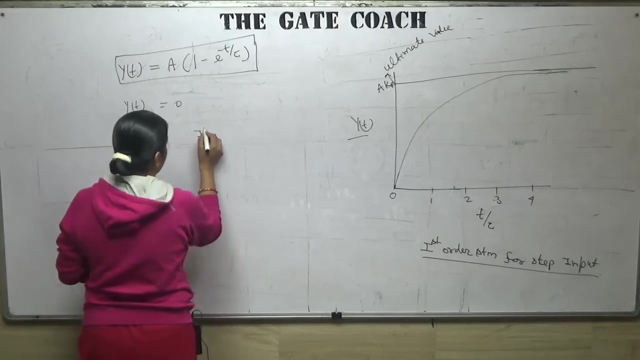 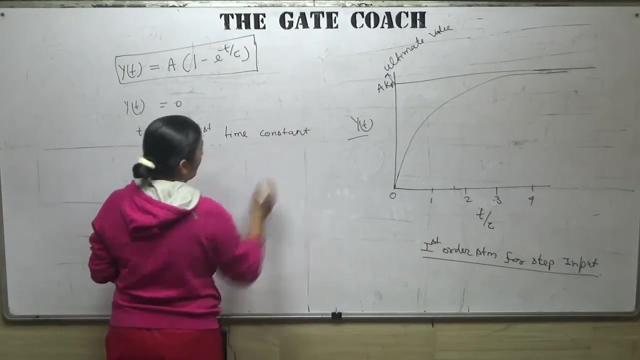 Curve will start from there: 1,, 2,, 3,, 4.. It will go like this: When t is equals to tau, We say this as first time constant. When t is equals to tau, We say this as first time constant. 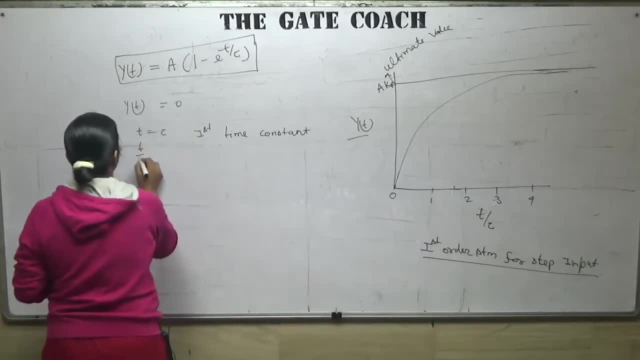 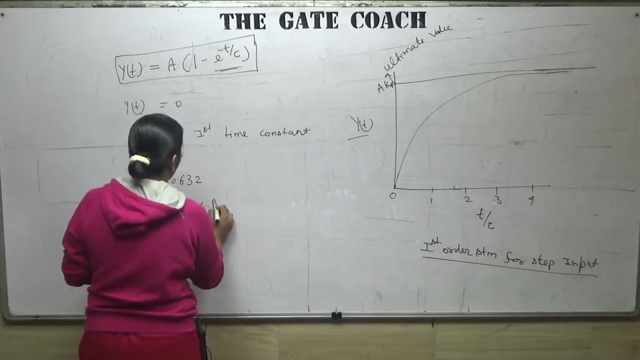 Means t upon tau will become 1.. Substitute value here You will get by t is equals to 63, 0.632. or if we write it in percent It will come like 63.2 percent of a. Or if kp is here, akp. 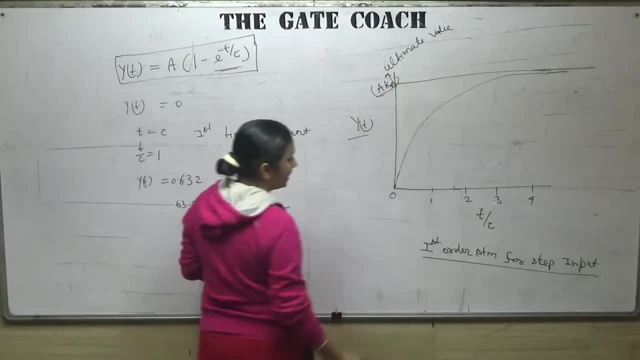 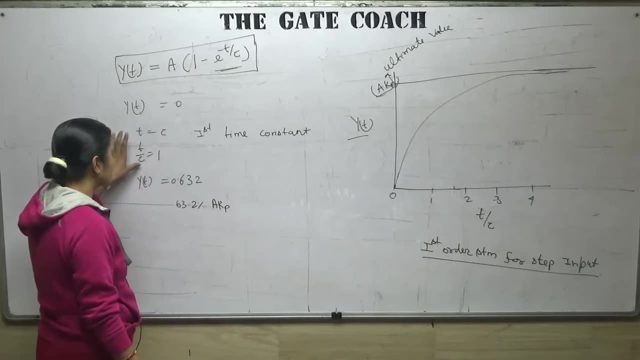 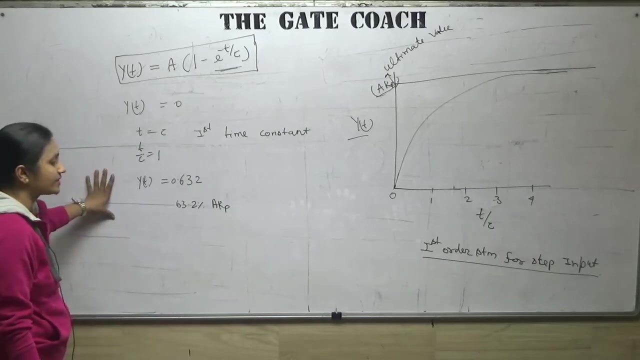 That will set it as 1.. ultimate value: ekp is nothing but the ultimate value. so from here, at first time constant, when t is equal, to write down this thing. this is important. it can be asked as a an objective question for one marks like, for the first time constant, how much value it will reach to the 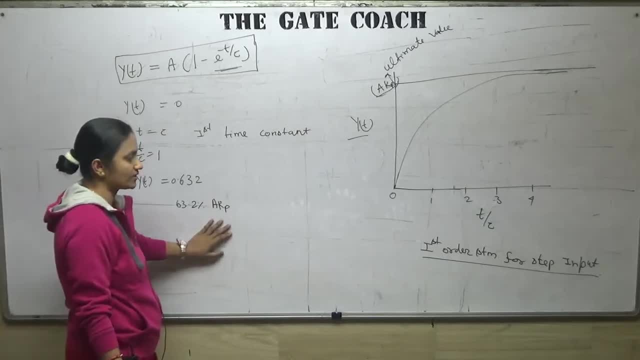 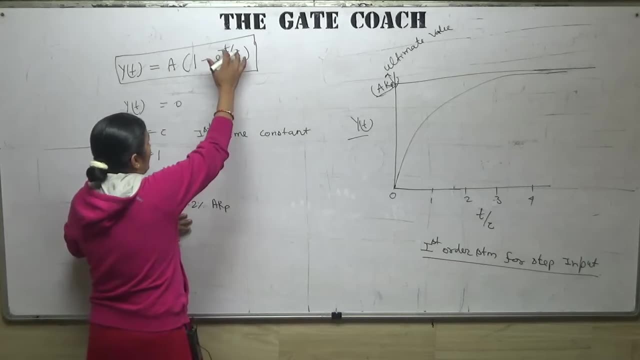 ultimate value, output will reach to its ultimate value for the first order system for a given step. input right, so it is 63.2 percent. write the value here, it will fire, minus one it will come something. one minus that value you will get is 0.632, something calculating your calculator. 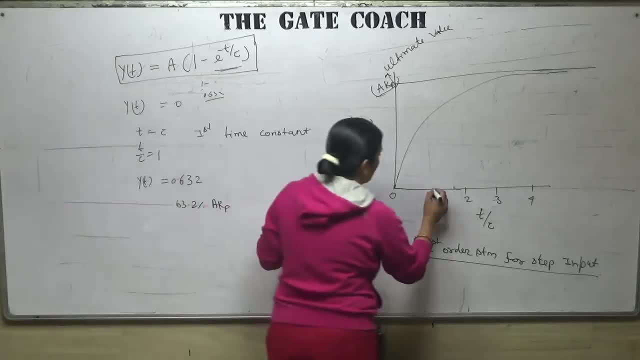 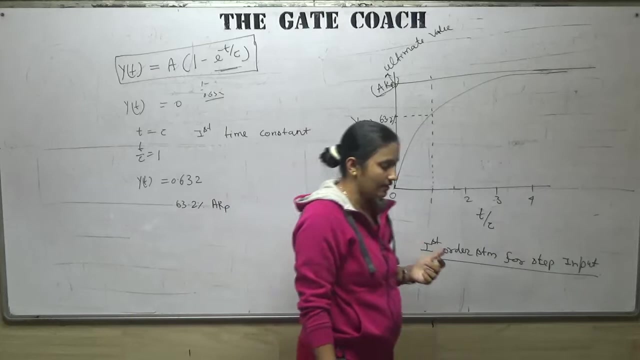 so, at the first time constant, at the first time constant, the output value will achieve its 63.2 percent of your ultimate value, that is, akp ultimate value. what is the conclusion of the equation from that conclusion, from that is that initially, this is the mathematical and what is, uh, practical? 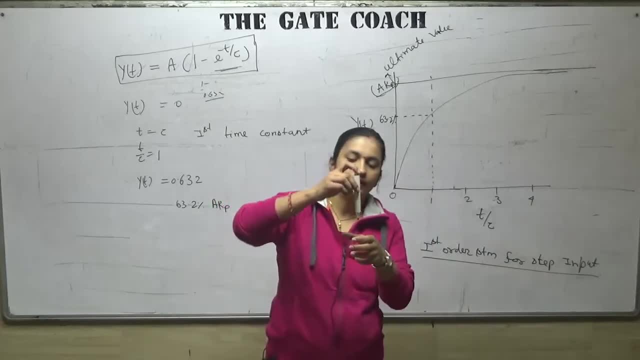 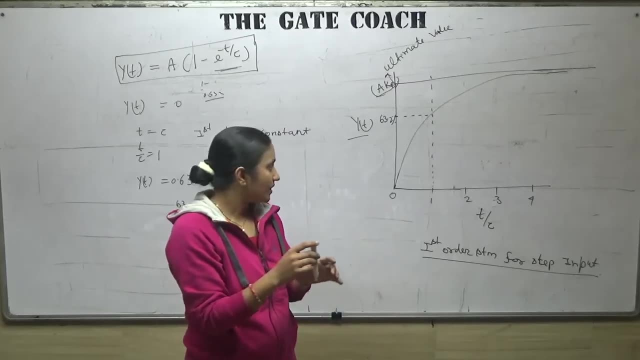 like your thermometer is there. you have put it into a water at particular temperature, like 100 degree centigrade. so initially it will. it will rise up to the temperature very high, because it reaches to 63.2 percent. why? because initially the driving force is more, that is, delta, t, the. 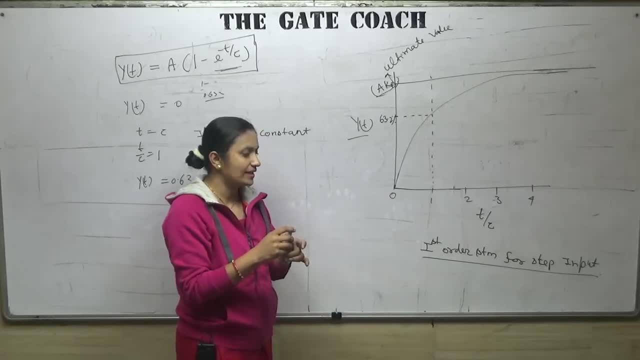 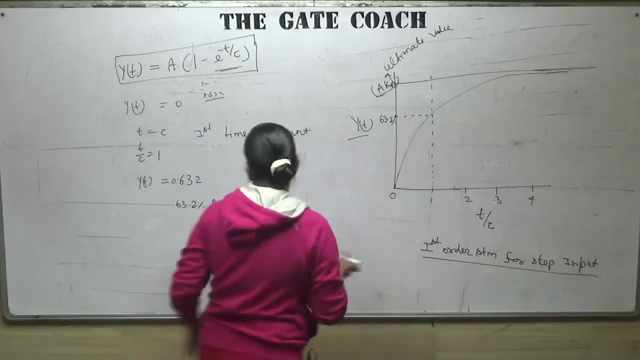 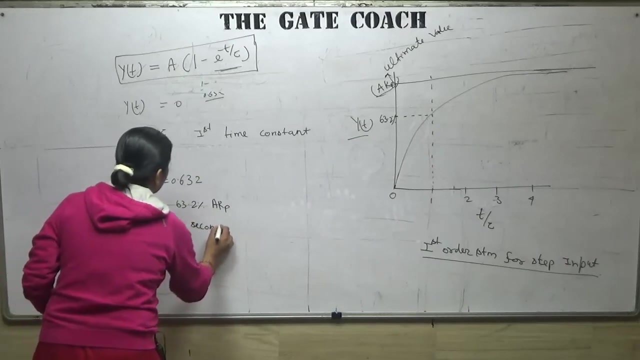 difference in the temperature is more, so that rate of heat transfer will be more right. so rate of heat transfer will be more means more amount of heat being transferred. initially, when t is equals to 2 tau, that is the second time constant. we say it as second time constant. 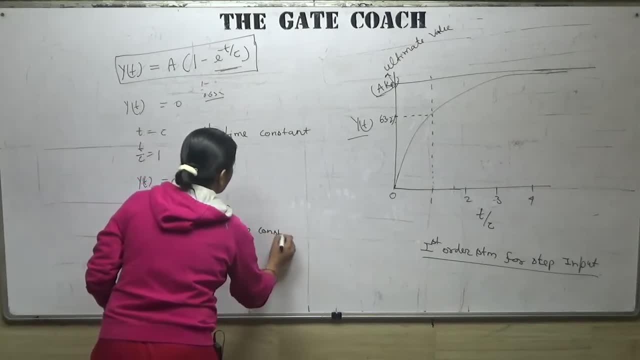 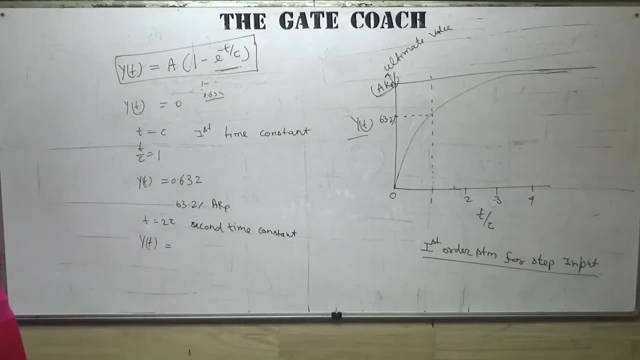 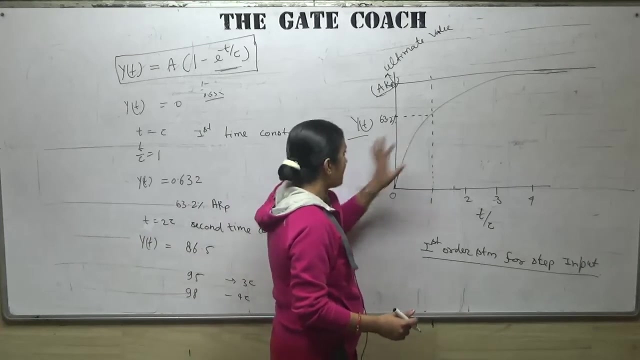 that by t will go to how much value value that by t will go to how much value- 86.5, then 95, then 98 for 3 tau and 4 tau which initially, when your driving force is more, more amount of heat is being transferred and as the time proceeds, we know the thermometer. 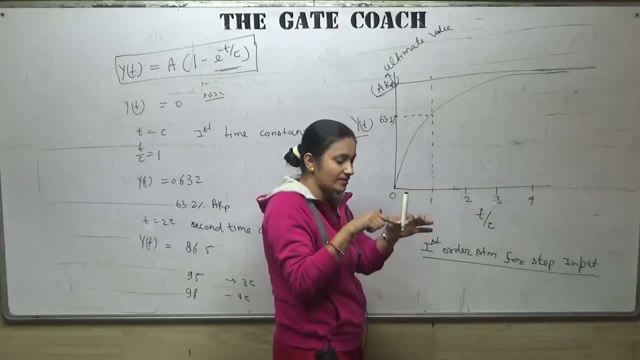 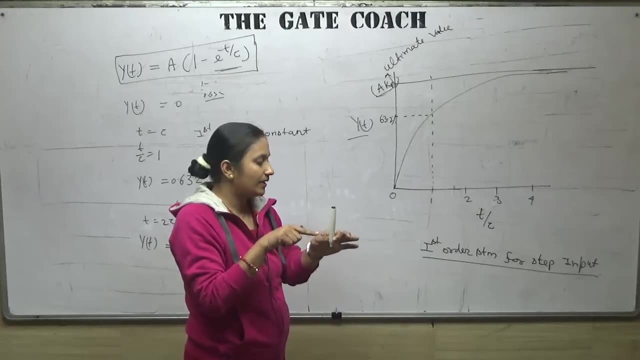 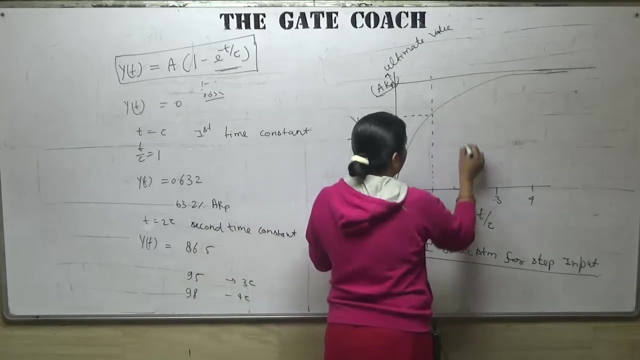 attains a particular temperature, the delta t difference will reduce. so the temperature and velocity in which we TALIESIN lamb to a particular temperature is as the temperature increases, that temperature may decrease because thermometer has attained particular temperature from that fruit. so it will take time, it will take, it will gain the heats at 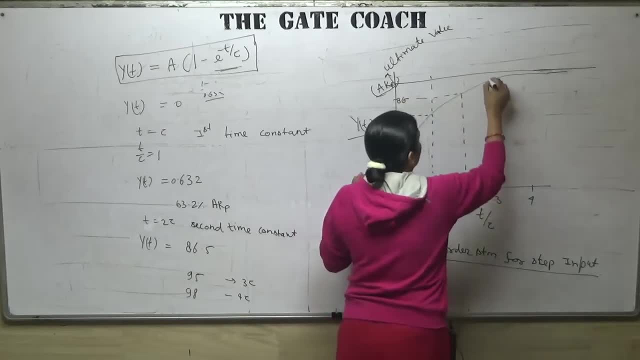 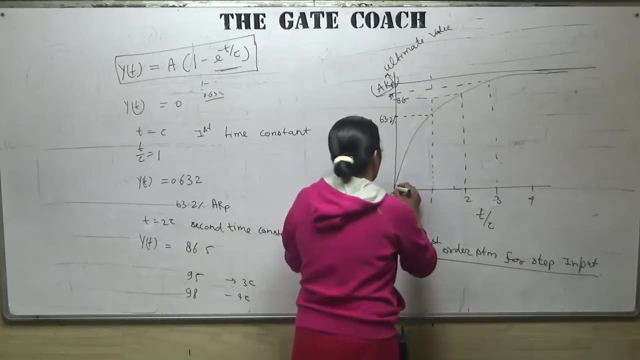 a slower rate. so it will so up to at the second time constant at 86 and after that 95 percent means maximum of the heat it will gain at its first time constant and if we maintain this, 0. So if we are able to maintain such slope then we can obtain the final 100 value at. 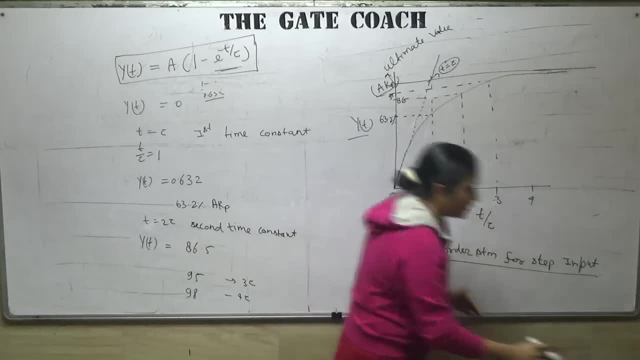 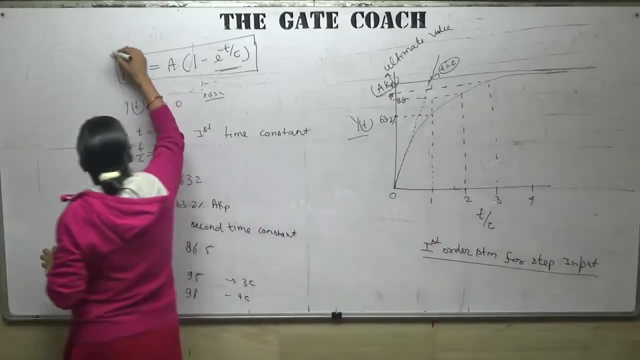 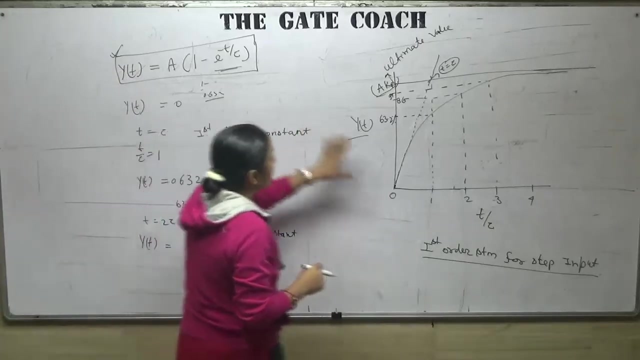 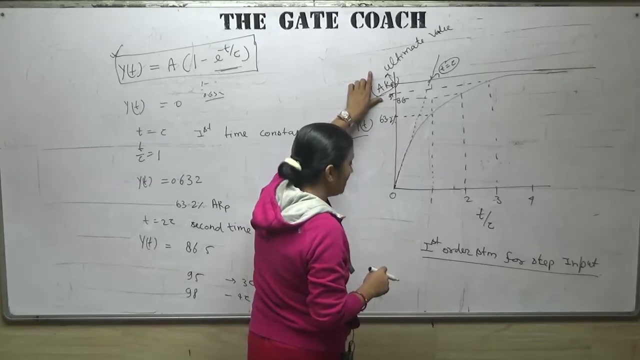 its first time constant, But practically this is impossible, But practically this is impossible. So this is the logic behind this formula and the graph explanation: right: At first time constant, the output will attain its 63.2% of its ultimate value, of its ultimate. 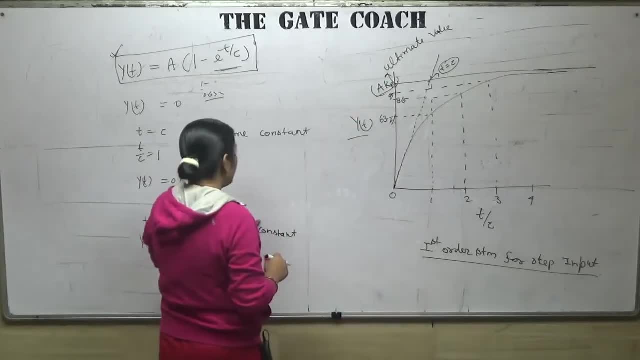 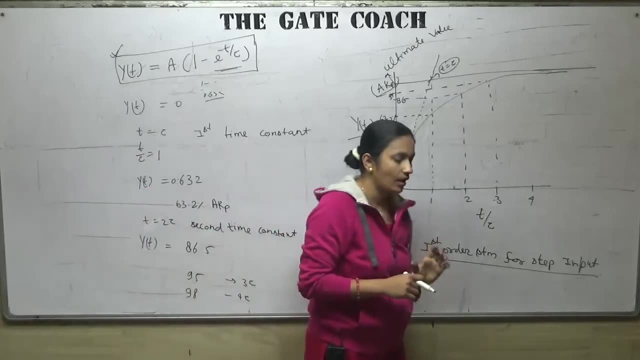 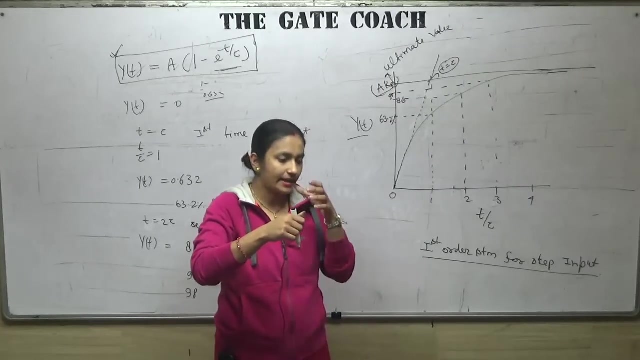 value right, And in second time, constant, it will go to 86%. Substitute t is equals to 2 tau. you will get this. And why this is so? Because initially the temperature difference is more means rate of heat transfer will be high, right. And as the time proceeds. 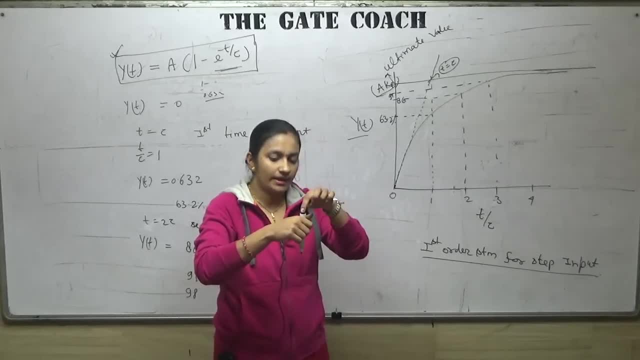 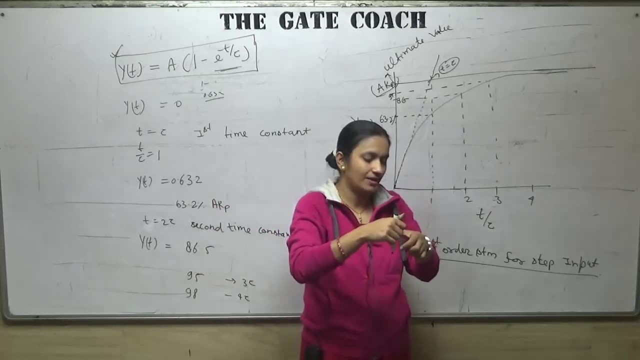 as the time proceeds, the thermometer will attain certain temperature In order to make it higher. for that, that, driving force reduces, means rate of heat transfer becomes slight slower as compared to before. okay, Now solve the question again based on this graph. 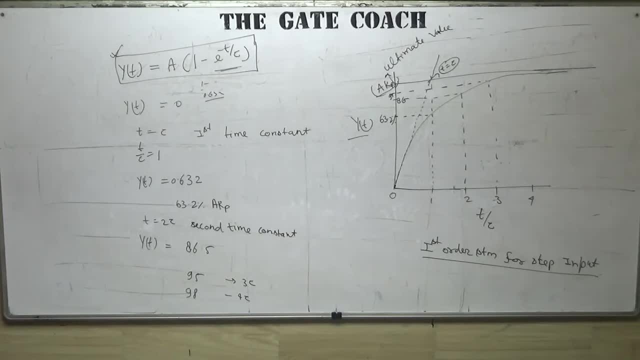 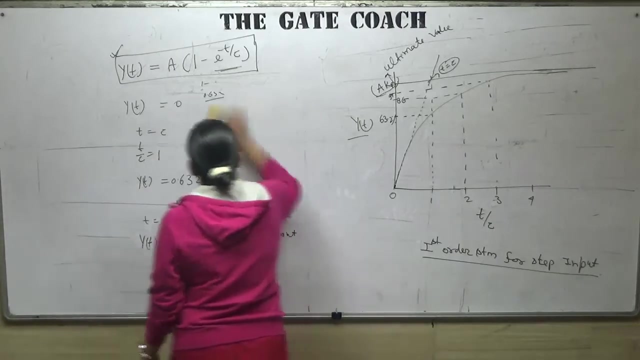 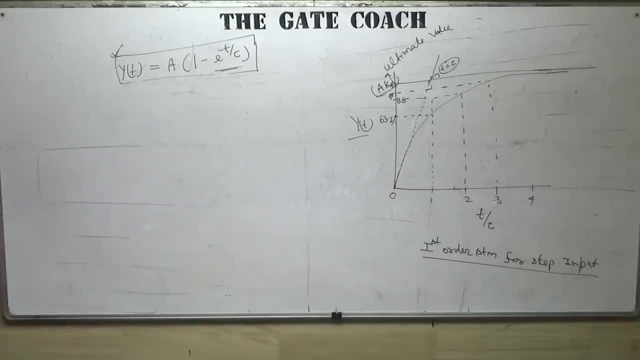 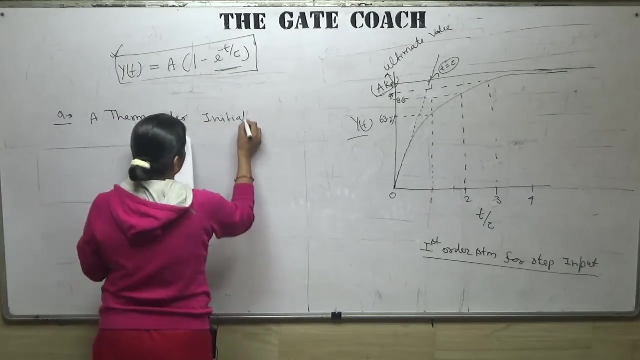 You just find what is y. What is y is what is given in the question. The question is: a thermometer, initially at 100 degree centigrade is dipped at. is initially at 10 degree centigrade, Is dipped at a temperature. veulent este ez. yi ayas per 아니 mater keen ki tau tau anay as a comma, JUNE 2012,. question 2: other than Mor, A thermometer divided by 10 or so byischalking at a str. multipl크 says even ludes at a temperature. 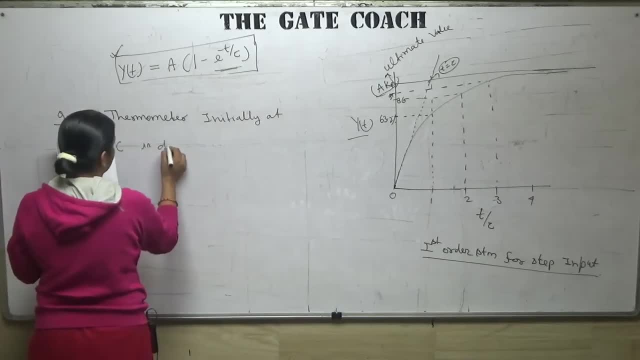 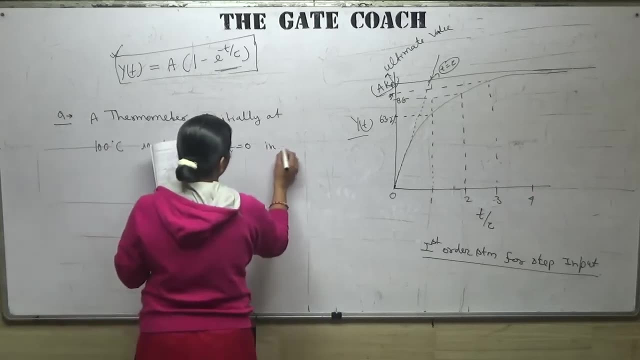 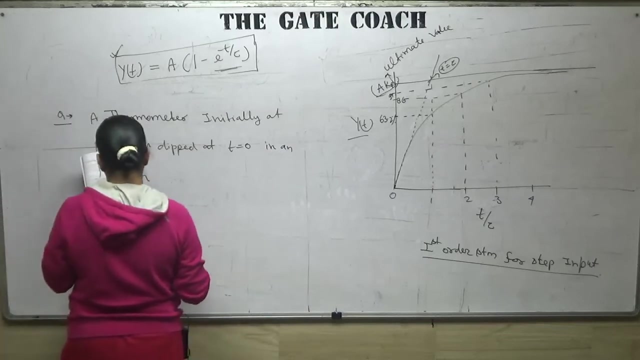 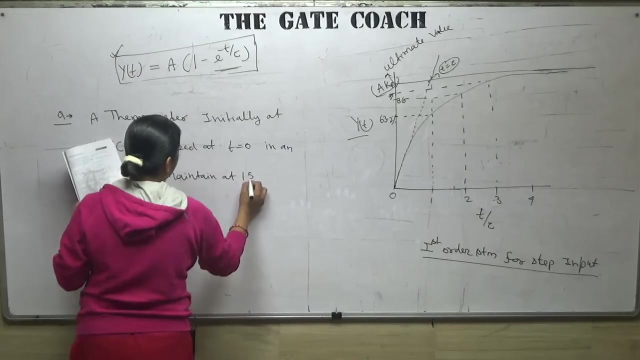 m c-1 is basal number, anay that it is save of energy not obtained from it. buf Parents are Очth These place things too. That may be because of numbers of number- estimates obtained. T is equals to 0 in an oil bath maintained at 150 degree centigrade if. 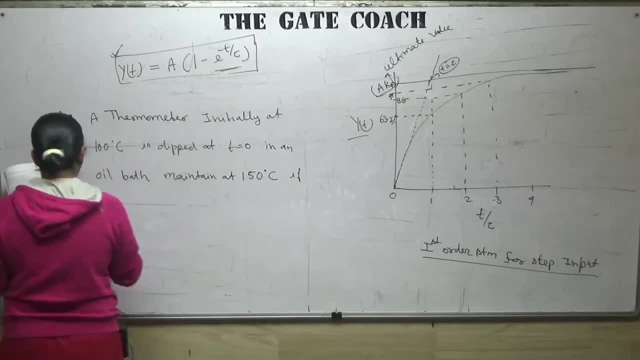 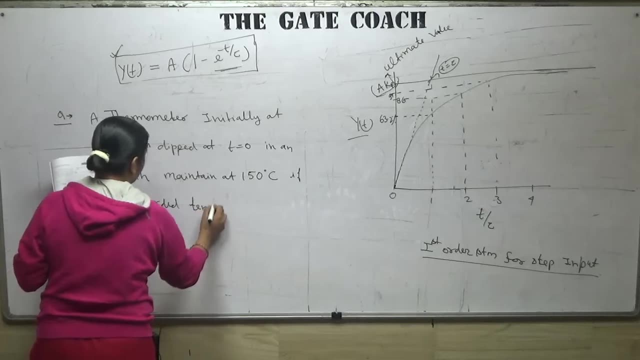 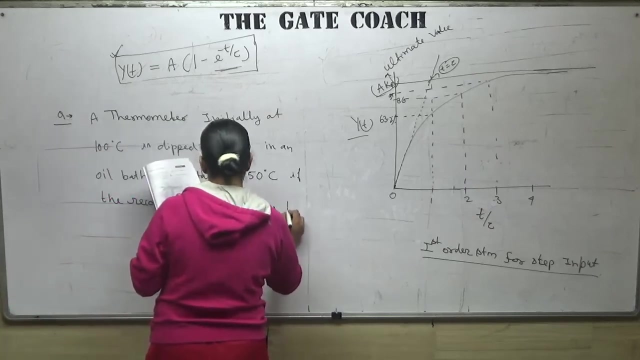 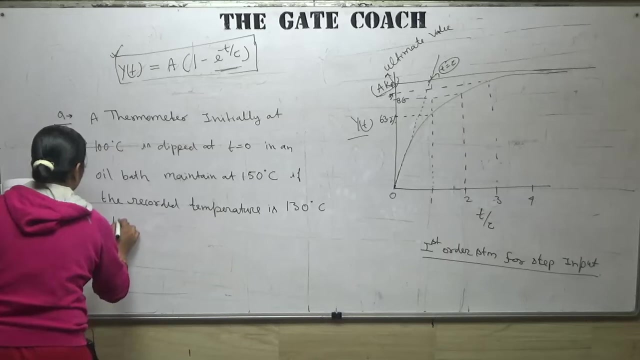 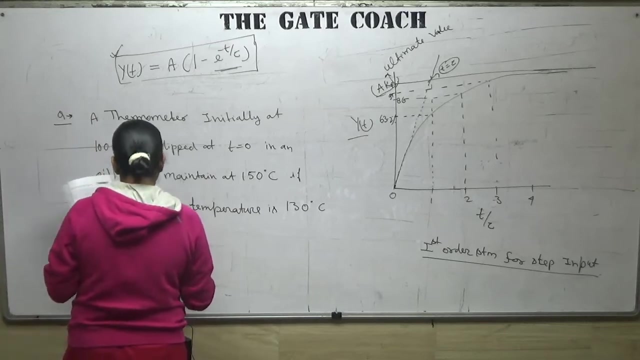 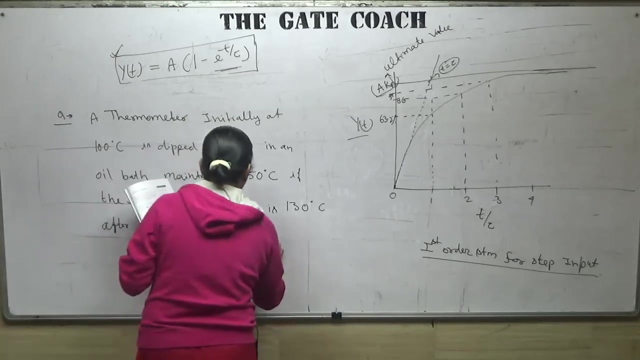 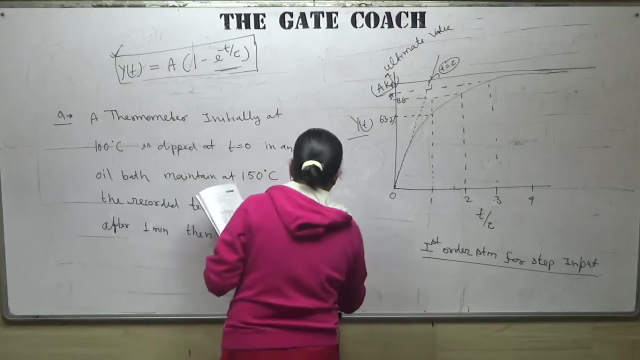 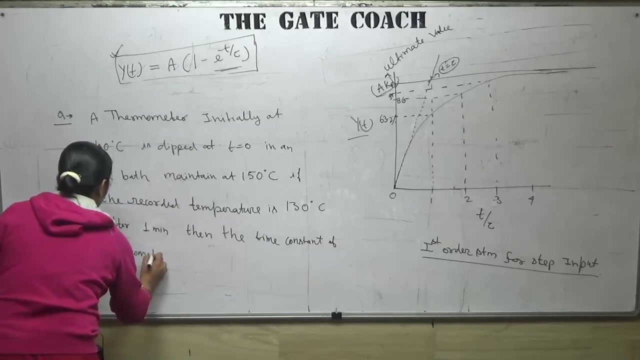 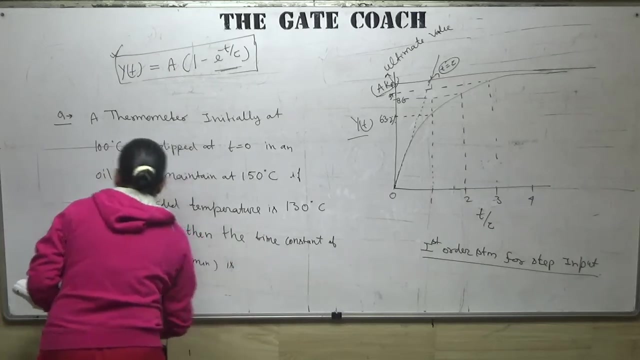 the recorded temperature. if the recorded temperature is 130 degree centigrade after one minute, after one minute, then the time constant of thermometer is. then the time constant of thermometer in minutes is the options are. this try to solve the question. this is all. the question one. 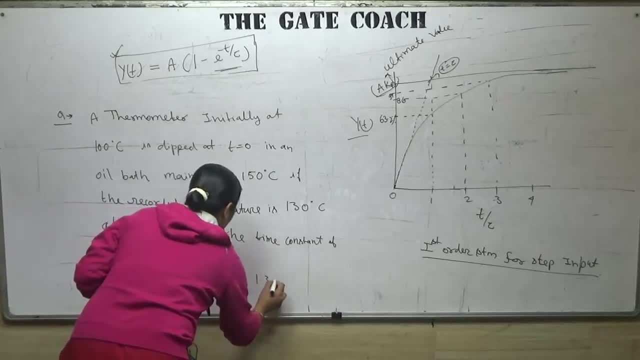 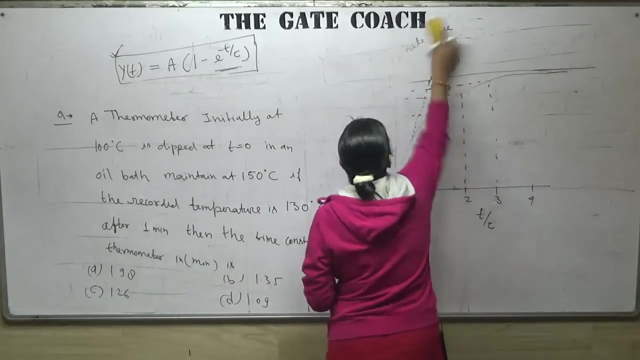 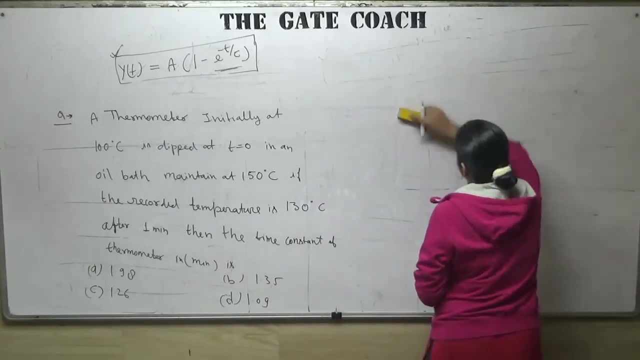 point nine, eight. option B is one point three, five. option C is one point two, six and option D is one point zero, nine. tell me this, all the question. tell me the value a thermometer initially acts, hundred degrees centigrade and is dip active. is equals to zero in an oil bath. maintain at 150 degrees centigrade if 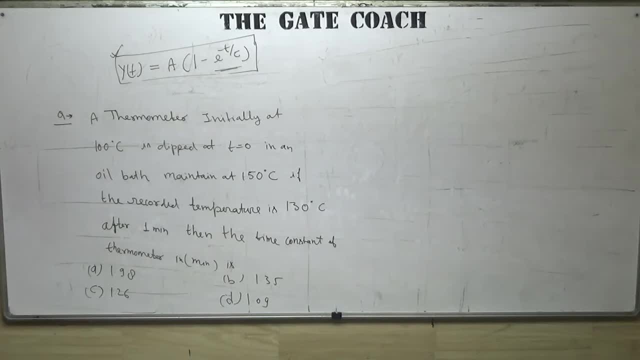 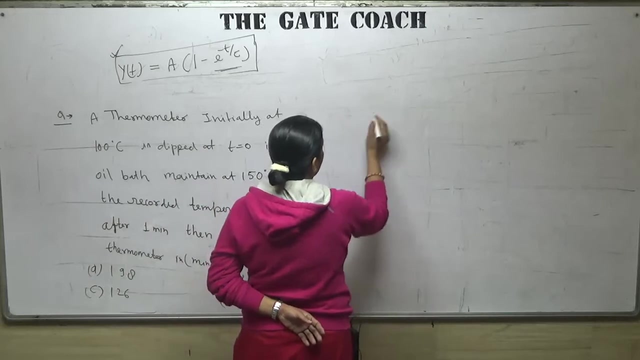 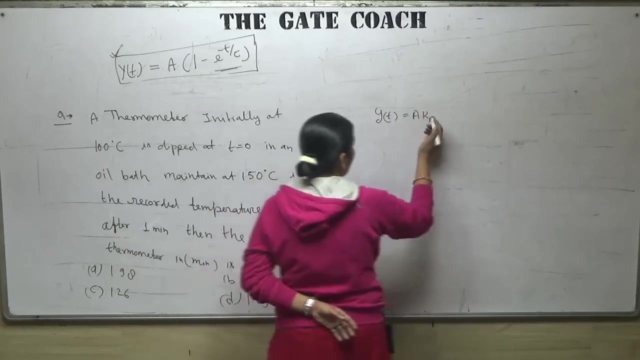 the recorded temperature is one 30 degree centigrade after one minute, then the time constant of the thermometer in minutes is yes. so what is the value of a here? which formula we will use by? T is equals to a KP, or simply a KP where KP is not given steady. 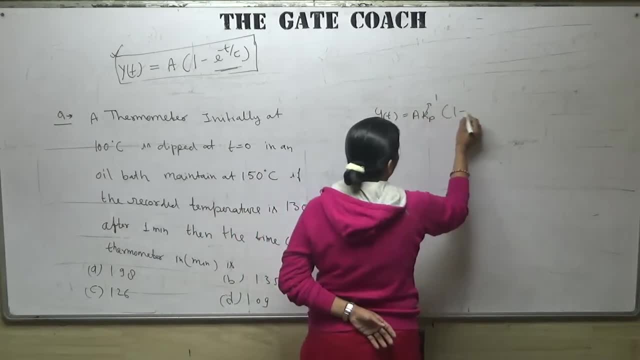 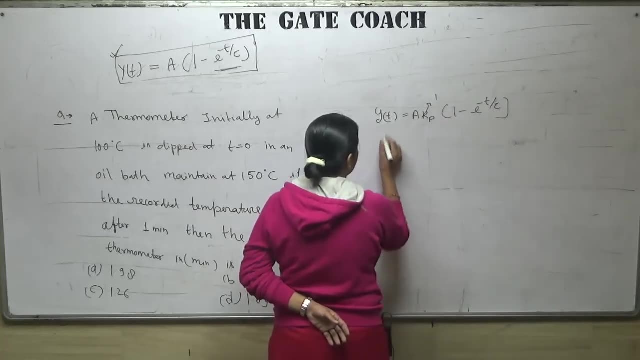 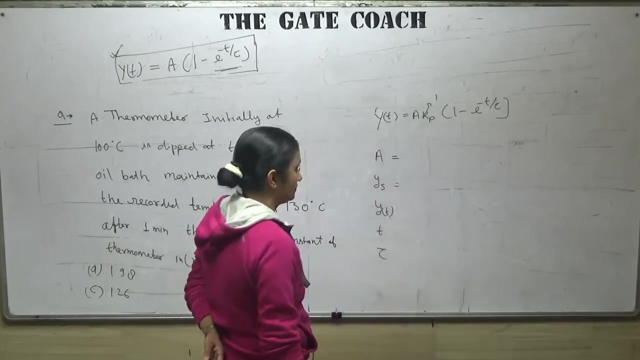 state gain of the process. take it as 1 into 1 minus e to the power, minus T upon tau. so what is the value of a here? what is the value of bias? what is the value of by T? what is the value of T? what is the value of tau? 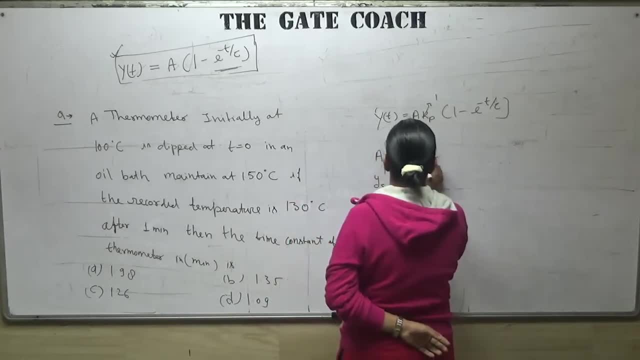 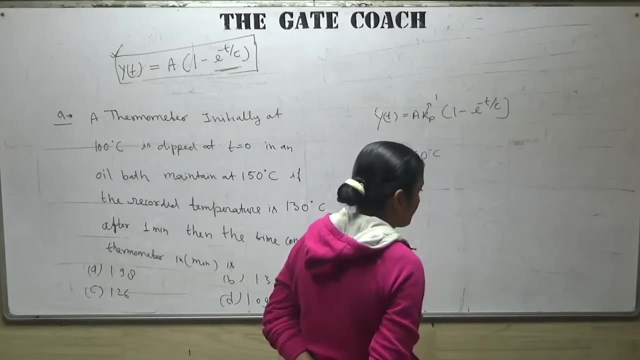 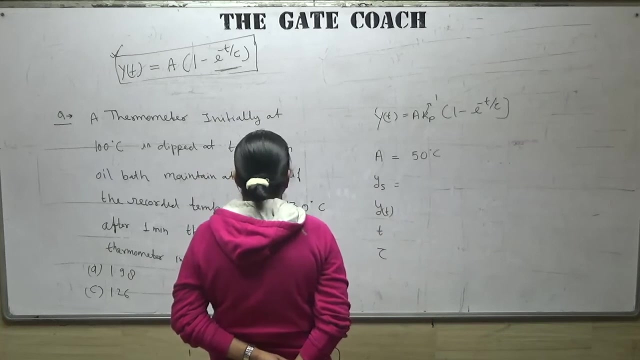 yes, a is 50. what is bias? bias is in easily. it is maintained at 100 degree centigrade. that is 100 degree centigrade. what is by T? that is, if the recorded temperature at is 130 degree centigrade after one minute means. 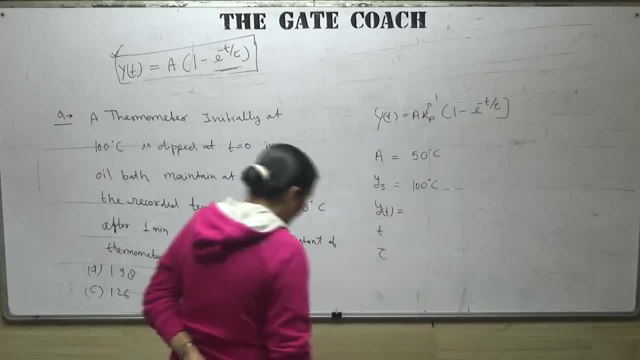 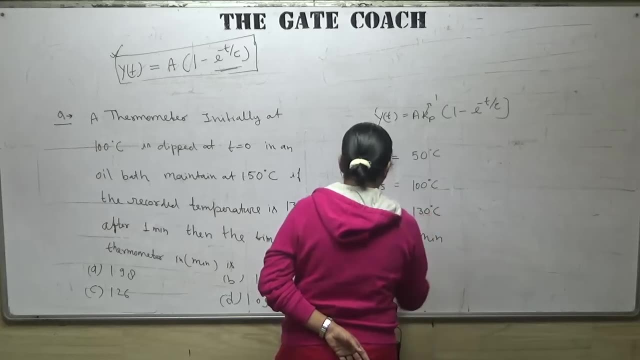 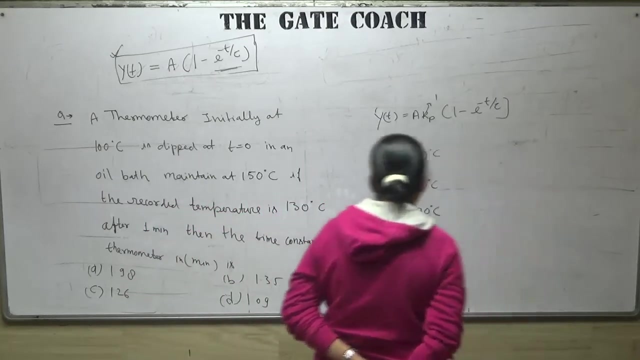 they have recorded the temperature after one minute. after one minute means it is time is given. a is equals to one minute, and what is? by T, 130 degree centigrade. then what is the value of time constant? so one is unknown. everything is known to you. yes, YT is 130. 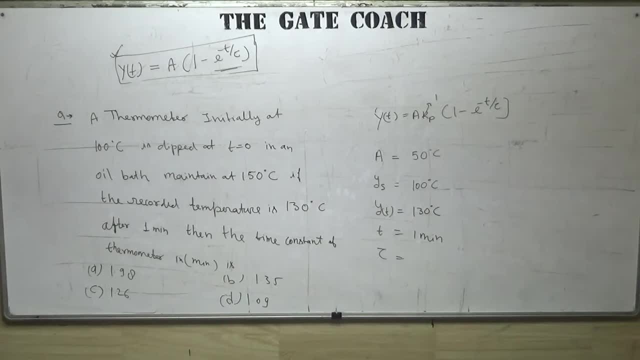 which option is correct? and by T that would be equal. the result of the. the answer is E, but because the value of T does not correspond the value of T or is equal to the value of T. but because the value of T does not correspond, the value of T does not correspond the value of T. 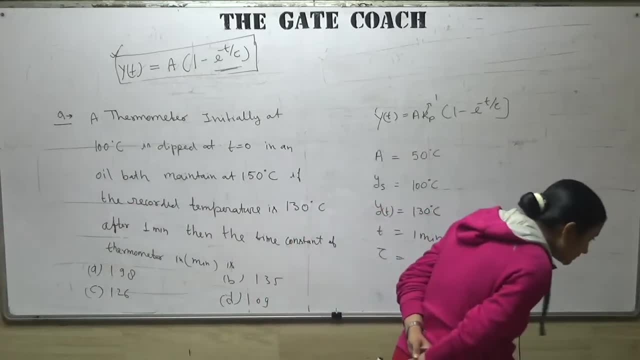 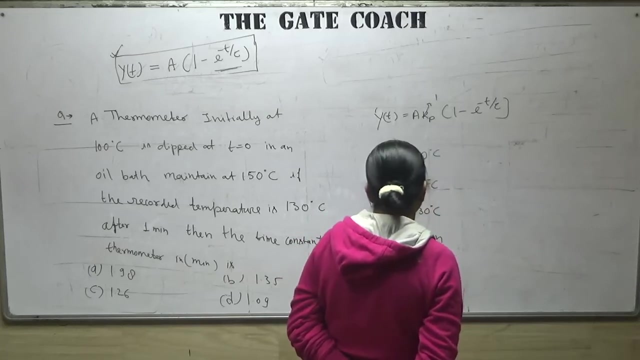 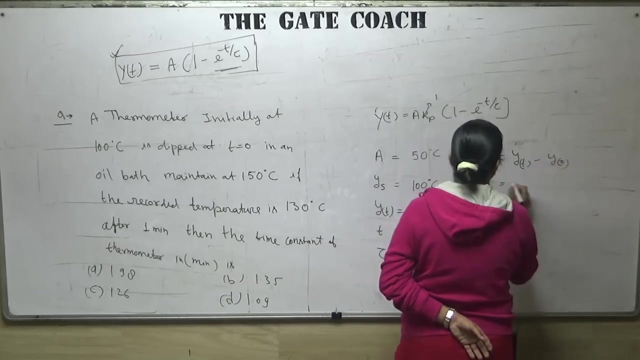 the value of tau is. so what is biotin? biotin is nothing but saturation. variable is small by t minus by 0, that is nothing but 130 minus 100, that is by as at steady state condition. so this will be 30 degree centigrade. 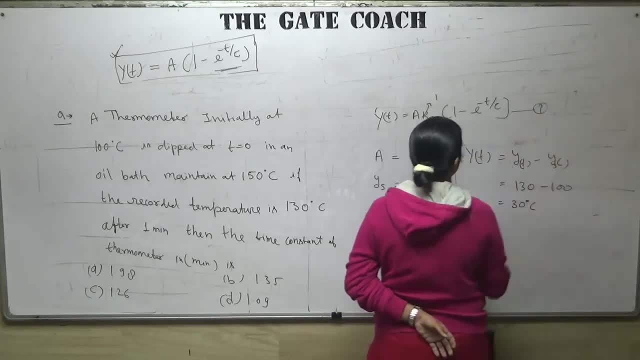 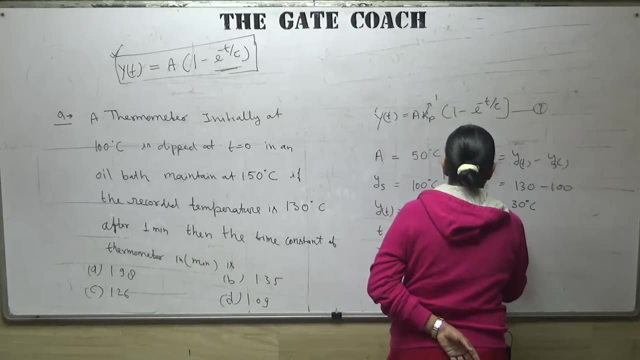 substitute values in this equation 1. that is the equation for the step input for the first order system. so this will come: 30 is equals to akp. the value of a is 50 into 1 minus e to the power minus t. t is given as: 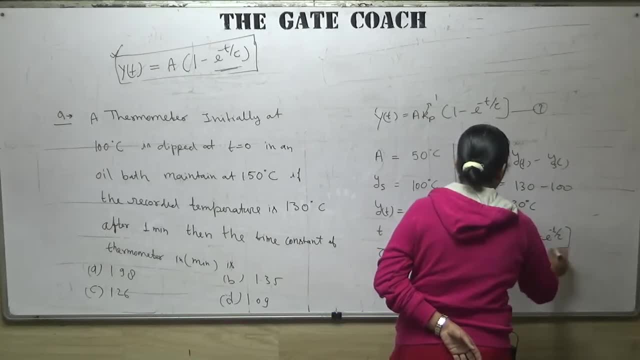 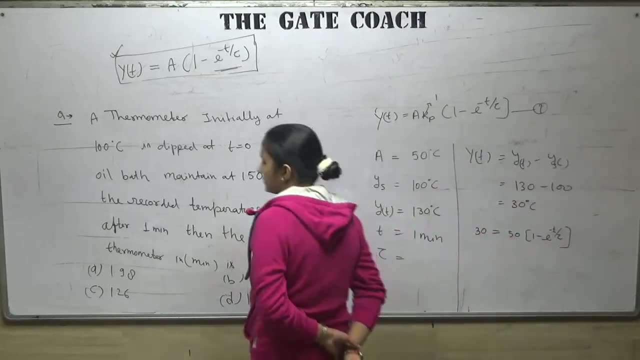 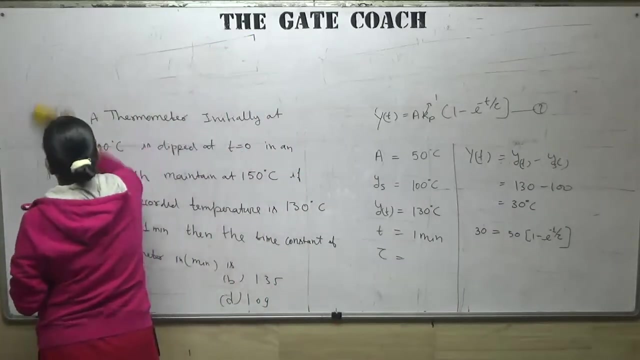 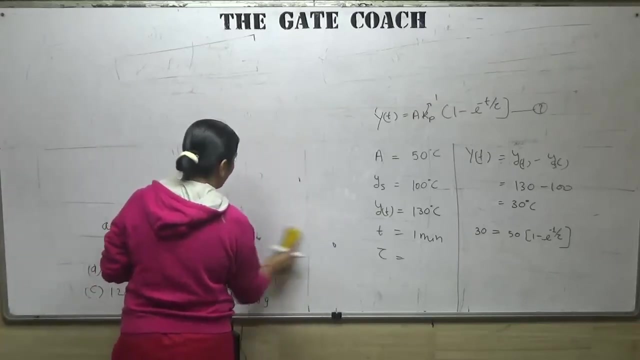 1 minute after 1 minute minus t upon tau. so this will come to you. yes, 0.09. option d is correct. yes, should I take the? this is: you must know what is the variation variable? what is time constant? what is time? what is initial steady state value. 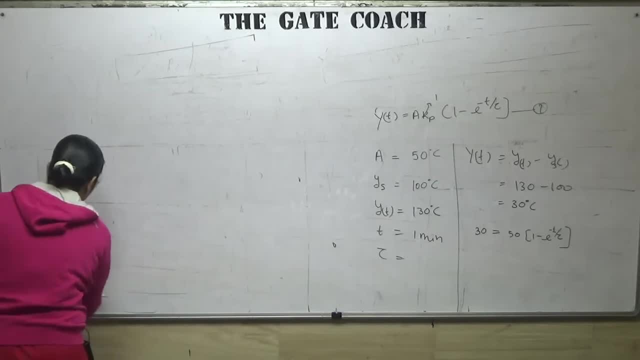 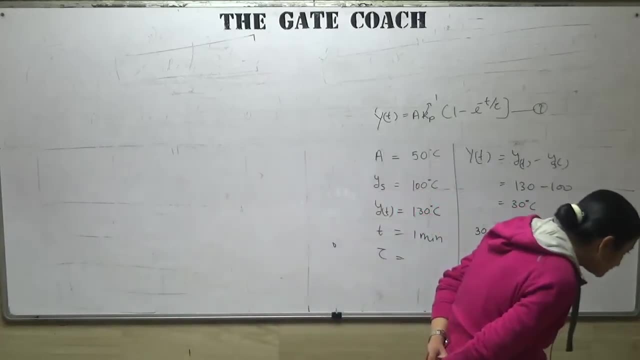 what is at any time, particular time, t value. you have to find out all the values and substitute in the question. you will get your answer. l n l n take l n take l n zero. zero get keno is equal to 0.50. OK, take l n zero. zero get keno is equal to 0.50. 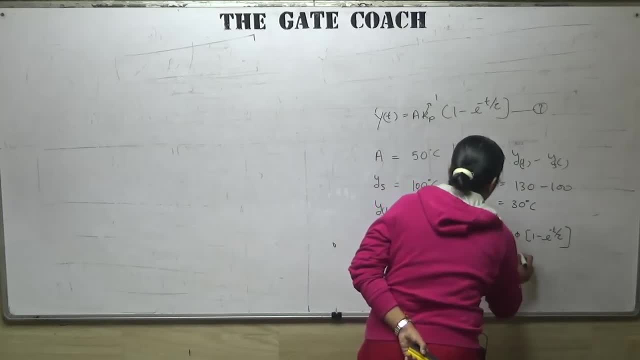 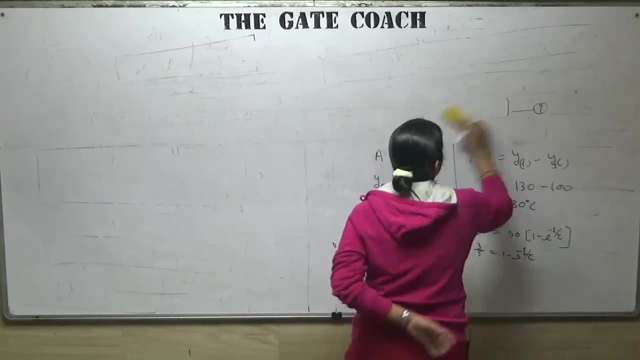 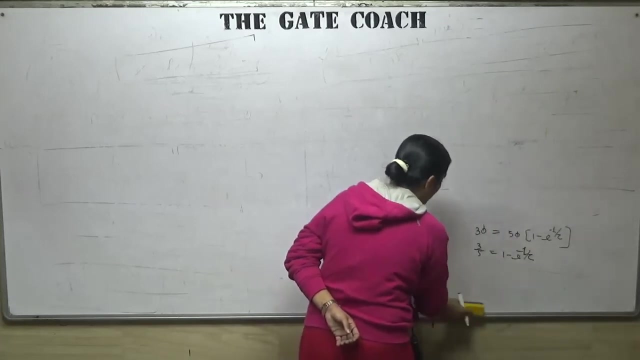 take l: n 0, zero, zero, get keno is equal to 0.50. cancel 3 by 5 is equals to 1 minus square minus 1 Y. so take L and both the sides. where log is needed, I will tell you the log until you take L. 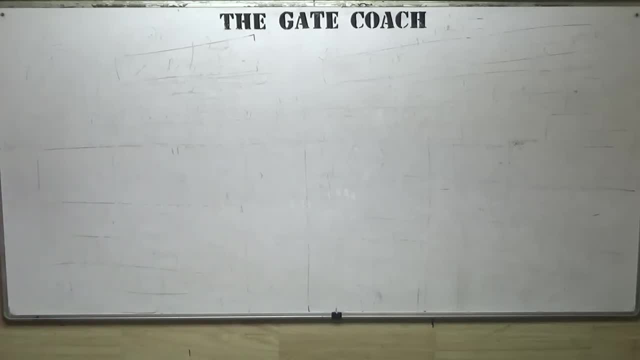 so that was the equation for the first order system I am giving you. I am moving towards the topic, first explaining you all the forcing function with respect to the first order system. right, I have just discussed. for the step input, write the formula for the impulse input. right, you have your. 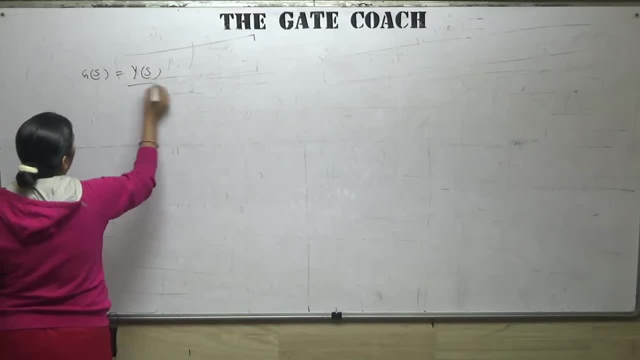 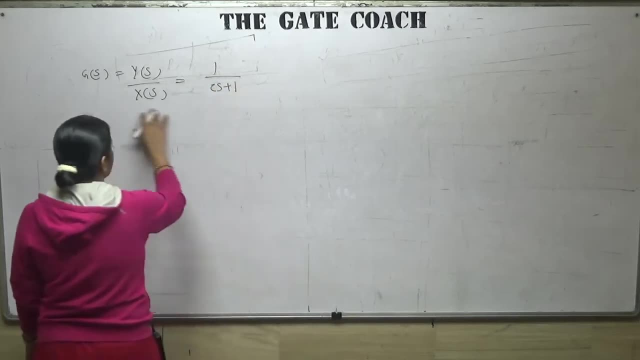 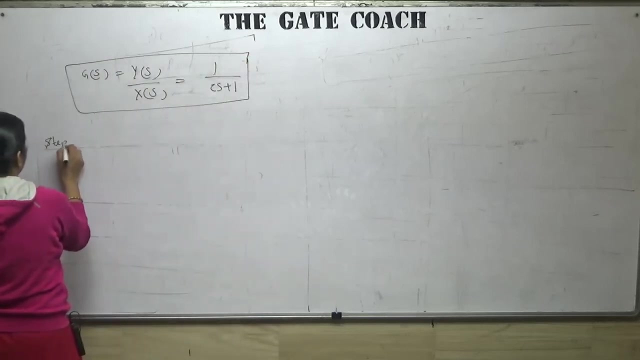 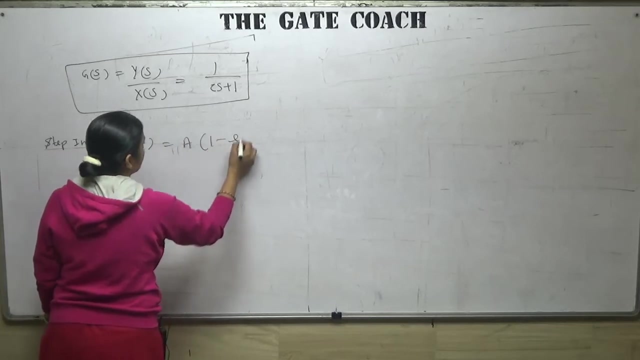 transfer function g. x is equal to Y s upon X, s is equals to 1 upon tau, s plus 1. that is, it is for the first order system. you have calculated for the stop input, step input. have calculated your by T is as a into 1 minus e, to the power minus T upon top. 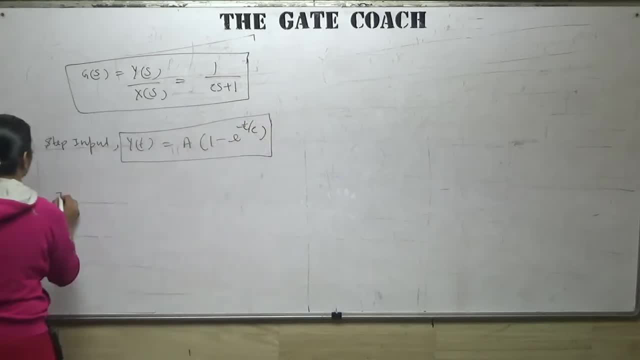 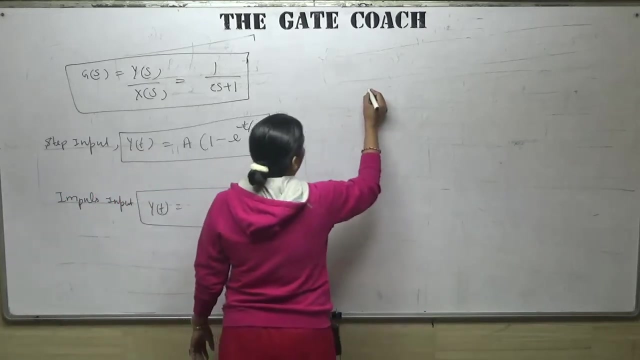 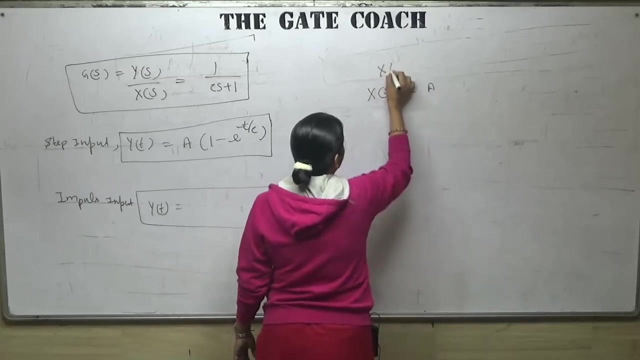 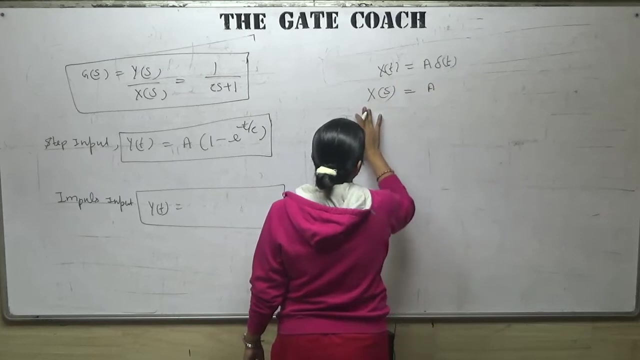 right. similarly, now you will vote for the impulse input. impulse input for impulse input. what is the value of by T? so look here: X s. what is the value of X? s for the impulse input? that is a, because X? T for the impulse input is denoted by a del T and Laplace of any del function is 1 and the Laplace of X T. 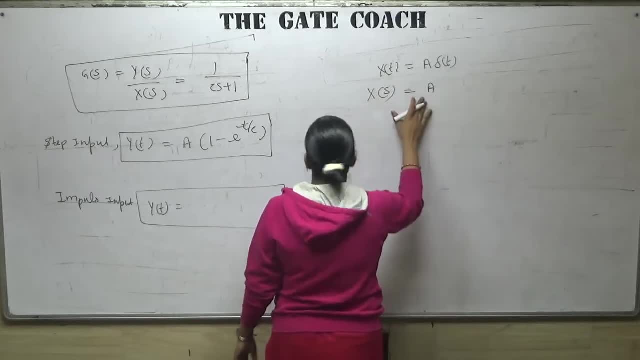 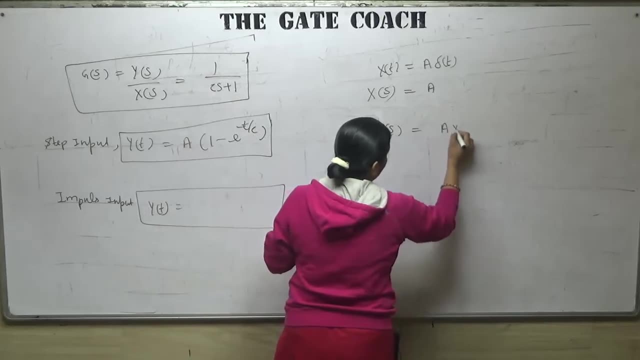 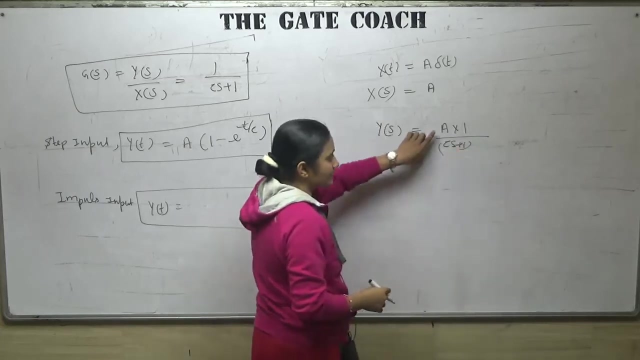 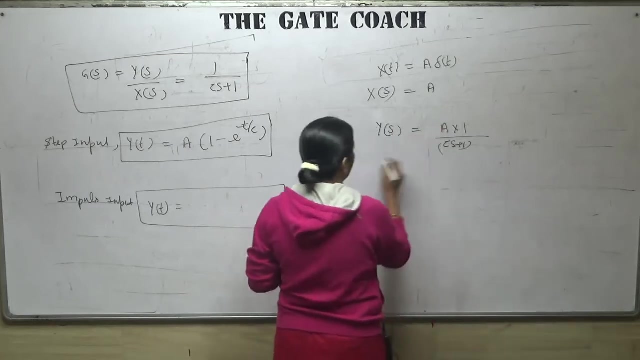 is equals to X, s is equals to a substitute. this value in your transfer function- then your bias will come- is equals to a into 1 upon tau s plus 1, where a is the magnitude of your impulse input, where a is your magnitude of impulse input, right. so take the inverse Laplace transform of: 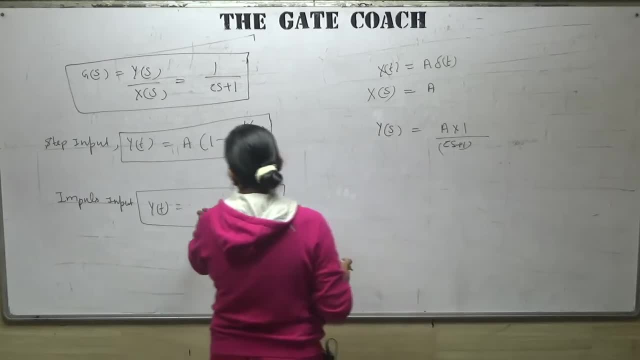 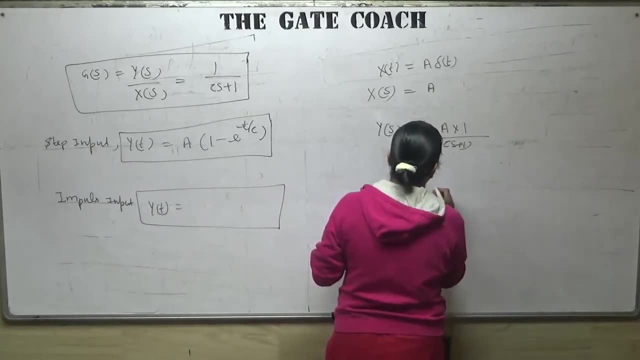 this you will get your. you will get the impulse input equation, so that equation will come, take it common as tau, or it will come like a Kp upon tau into e, to the power minus T upon tau. that is the inverse Laplace transform. or if Kp is not here, so you remove here Kp. if Kp is given to you, then 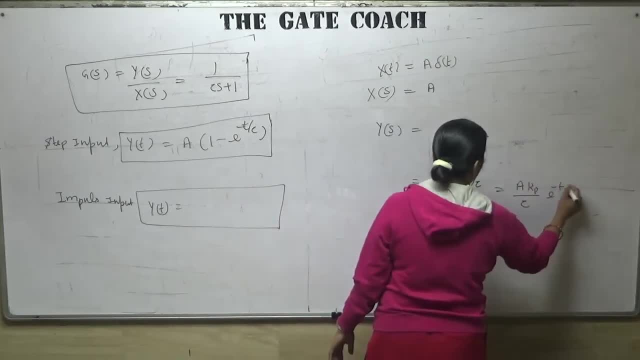 it will be a Kp upon tau into e, to the power minus T upon tau, because from here you will take common as tau. it will come as s plus 1 upon tau. s plus a is nothing but e. to the power minus a T minus a T is nothing but 1 upon tau into T if you are taking inverse Laplace transform. 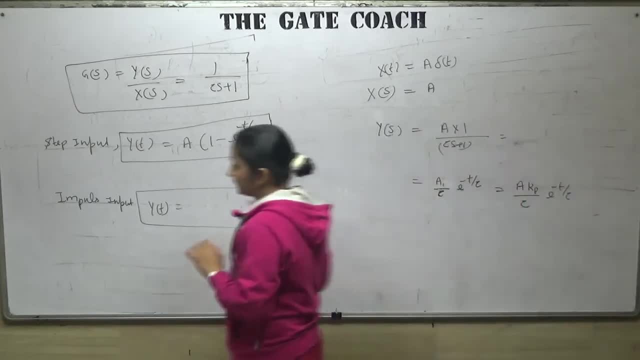 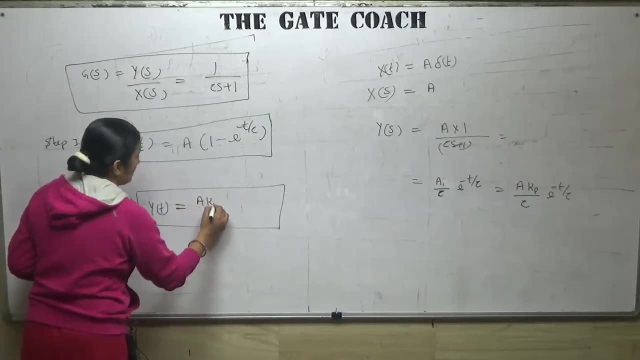 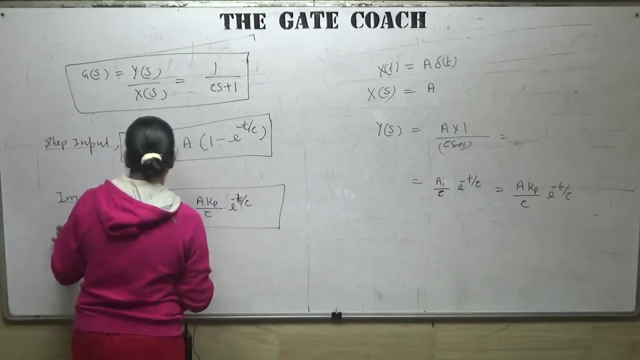 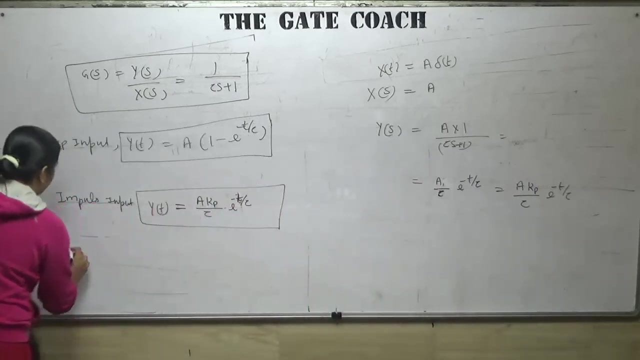 inverse Laplace transform. so this will come like this. so the equation for this is: a Kp upon tau into e, to the power minus T upon tau. that is for the impulse input. that is for the impulse input, similarly for the ramp input. you, you BruItalım. 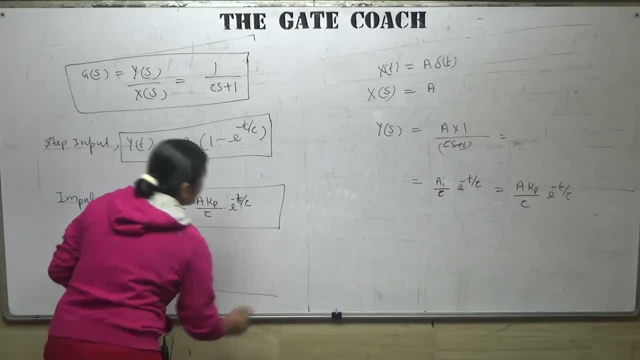 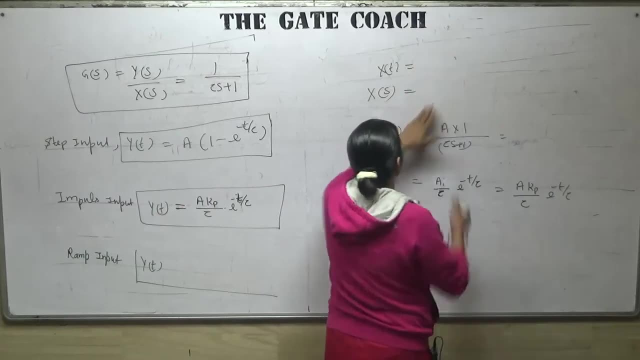 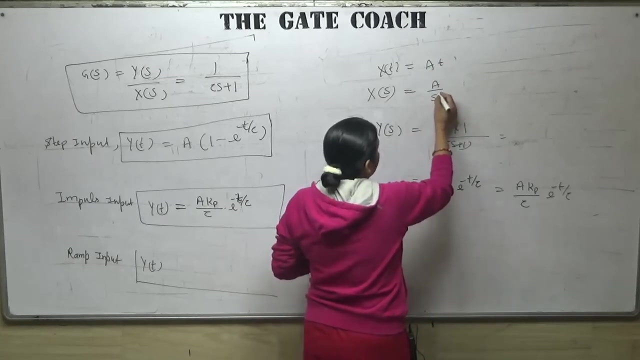 for the ramp input. what is the value of my T right? we know for the ramp input for operative inch onion. we have discussed what is the ramp input. ramp input is denoted by a into T and the Laplace transform of this is a upon s square. what is a here, here? a is this: law. here is the slope of the curve, this is what ith, this is the slope of a's curve plus t its the Citriol situation that we have discussed here. the slope of the curve, this quedarly breaking terms into twothe Å is plot answer, which is A times both positive tangôi as positive 2, and we have the permise of the Web S and minus Super ف, ta and minus C-2 here, all of them, which means that by settling theirabor, to put them like in between the curve and reducing the curve, this would be equal to J s Moscow, the neo S square, which means that if we take exactly exactly what is Natomiast, the simple motion of this bike, as we refer to latent ah. 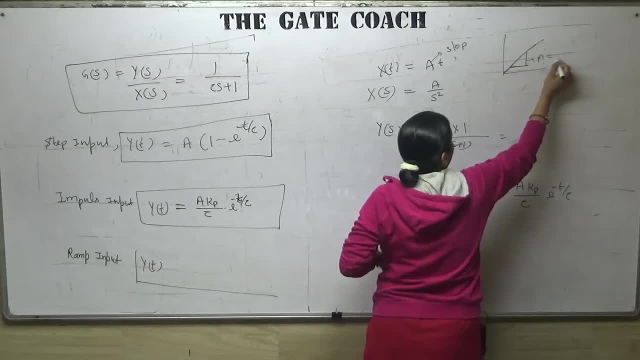 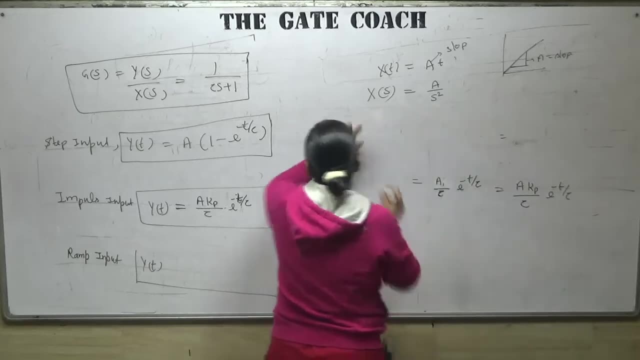 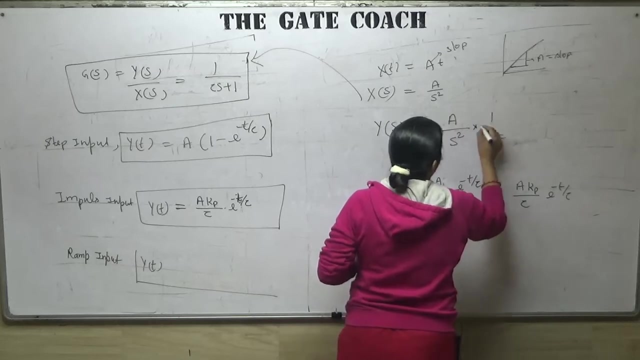 this one is a, that is slow in case of ramp input. xs is a upon s square. then you substitute this xs value in this, your laplace. transform the transfer function for the first order system, that is, your bias, will come, like a upon s square, into 1 upon tau s plus. 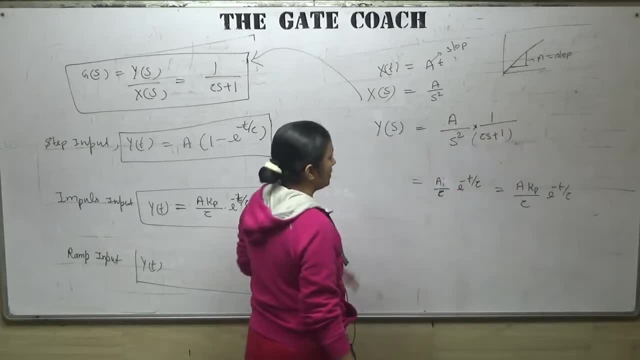 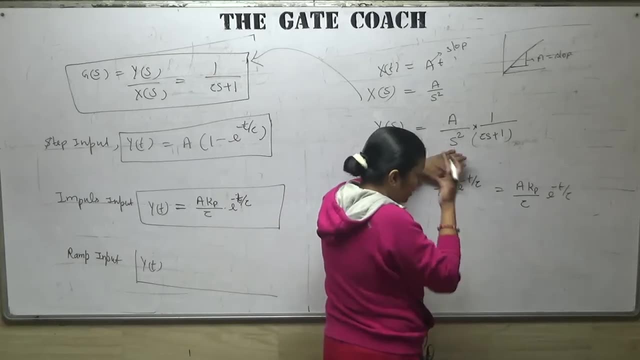 1. right now this equation comes like quadratic equation, so you have to take either quadratic power or you can say linear: uh, repeated roots s square is there same roots, same two roots. so solve this equation. take the inverse laplace transform of the equation, then you will. 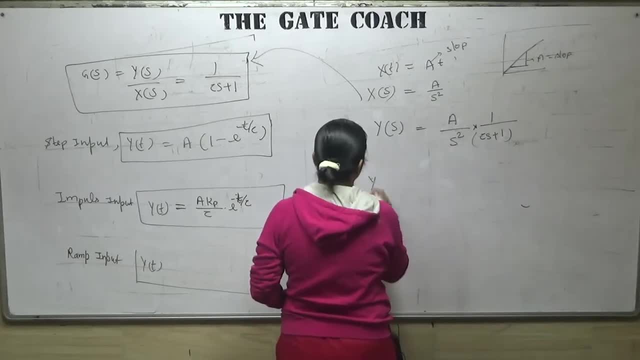 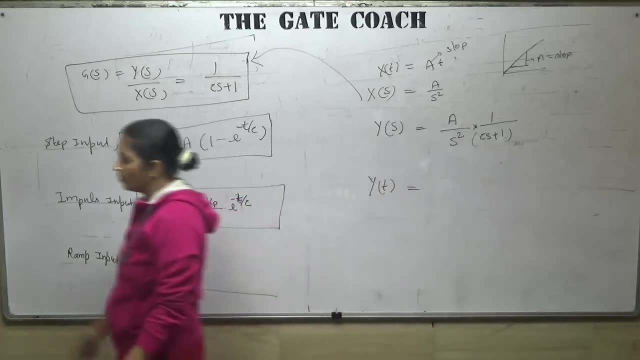 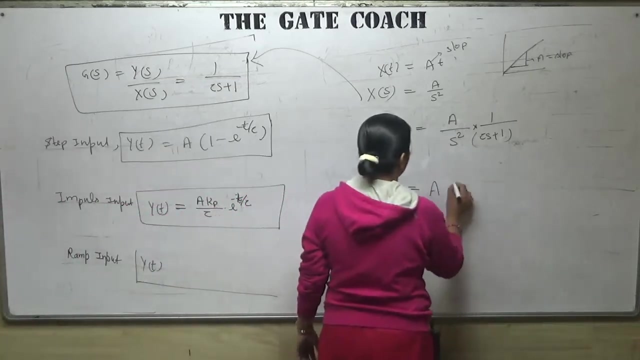 get the by t. take the inverse laplace transform of the equation, then you will get the by t transform of this equation. you will get YT. I am the writing it directly. if you solve, you can solve it. it is not quite up. that is a into T minus tau into 1. 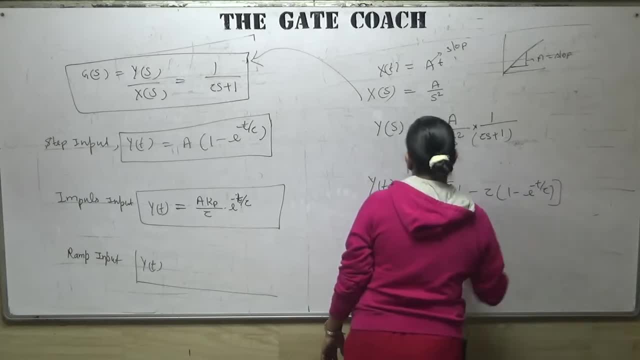 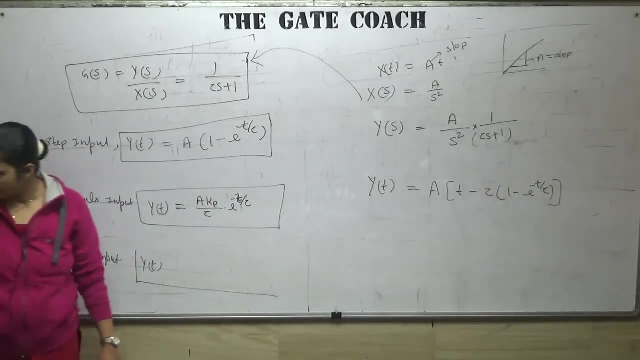 minus a to the power minus t upon tau. this is the response equation for the ramp input given to the first-order system: T minus tau into 1 minus e to the power minus t upon tau into a. escape is given here. you can write it here: escape. 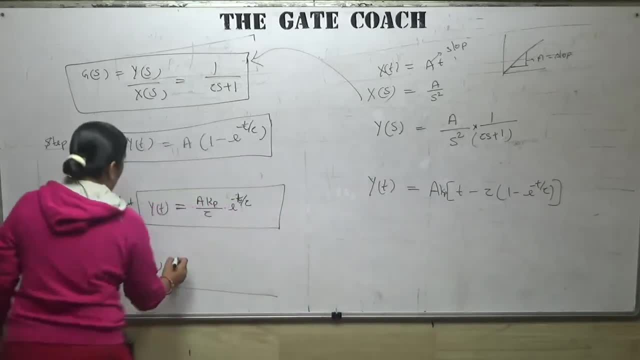 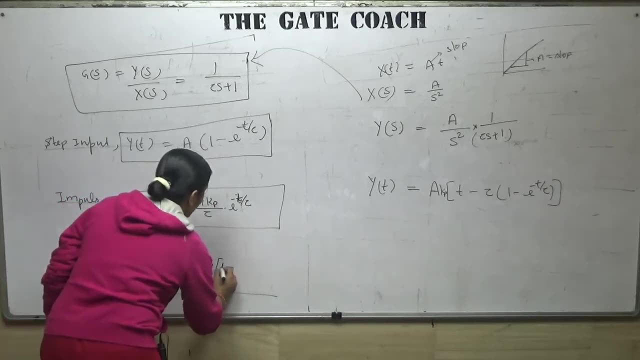 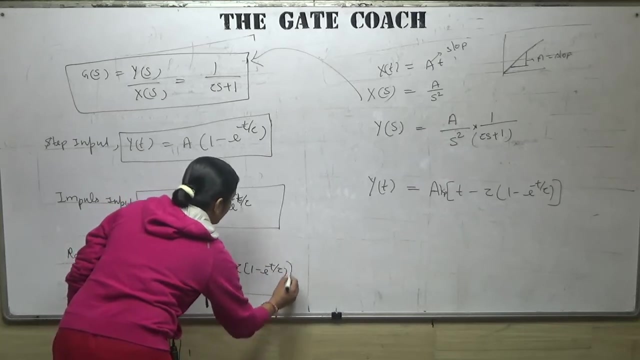 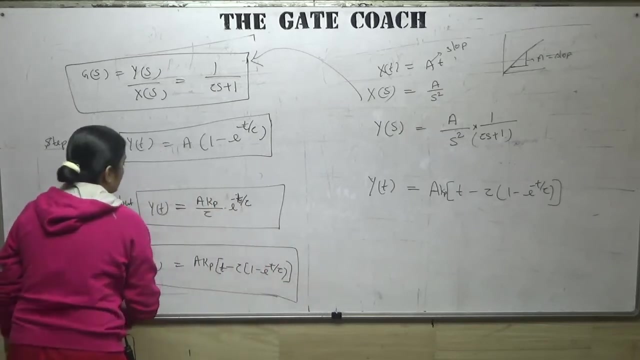 you also. so for the ramp input by T is equals to a KP, into 1 minus, into T minus tau, into 1 minus e, to the power minus T upon tau. this is the equation for the ramp input for the first-order system. most of the questions. 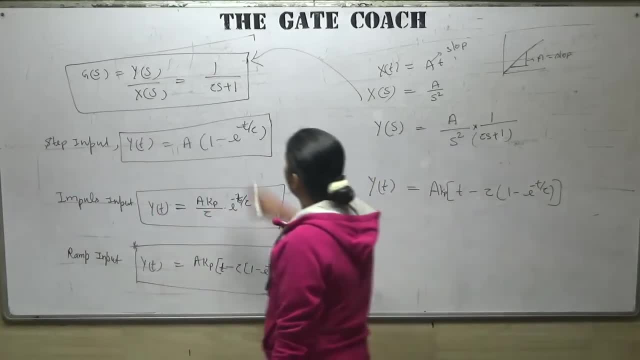 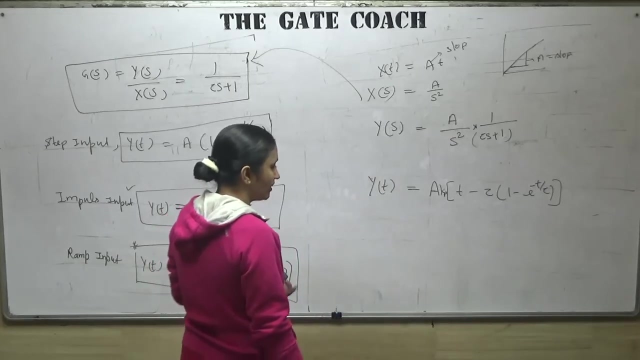 that are being asked till now is directly based on your step input and your input is directly asked for the formula, and ramp input is asked like graph-based. you have to calculate the slope, like as we have previously solved one question, so this is for the ramp input. 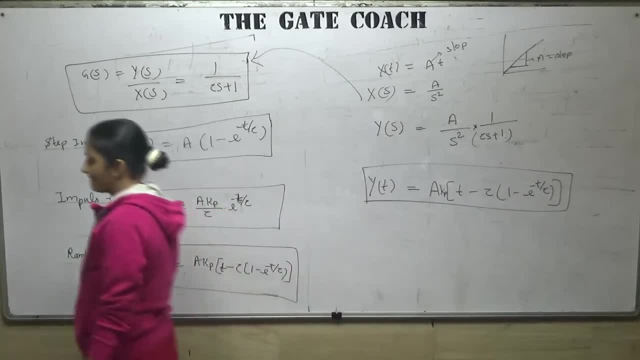 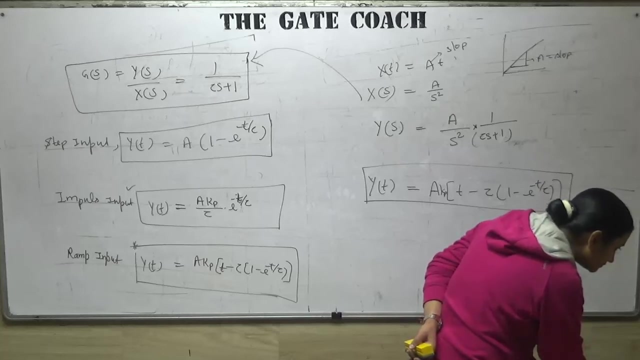 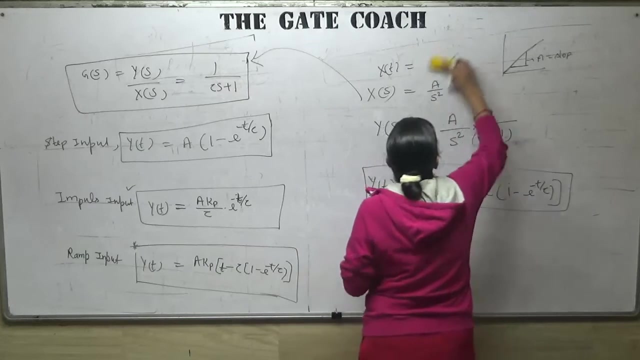 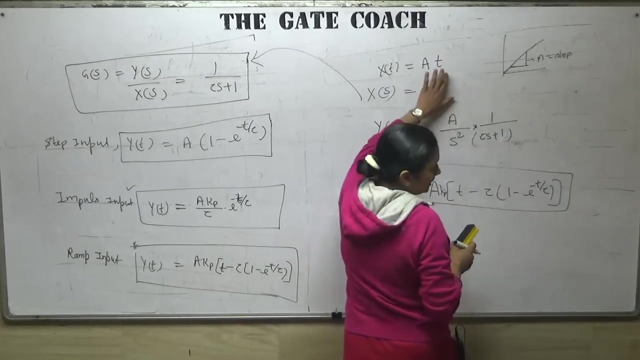 this one is for the ramp input. ramp input, or we can say the linear change. the another one is the sinusoidal forcing function. you xt will be akp, no, no, xt is a into t. what the ramp input, xt, is equals to a into t, means increasing linearly bit time t, our ramp function, also known as a linear function, 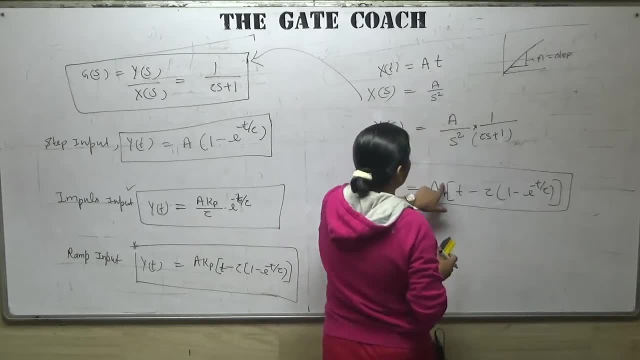 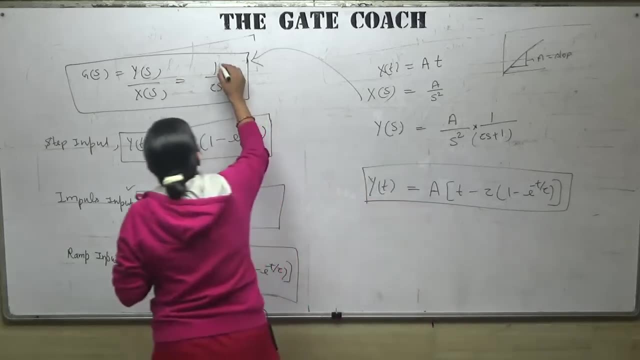 linear input right at kp is the steady state gain for the process. if it comes in the process that we have discussed that, it will come only here. kp will come here only in the transfer function for the process. right, if we are considering kp here, you can write kp here. 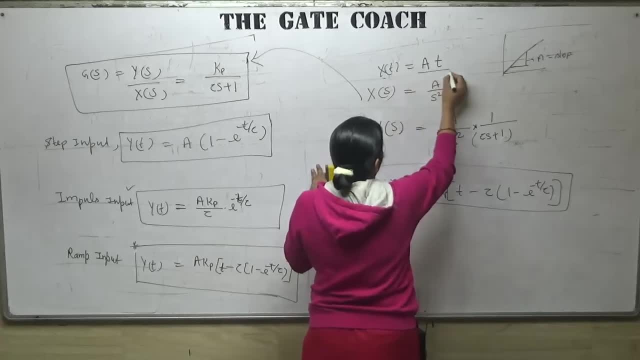 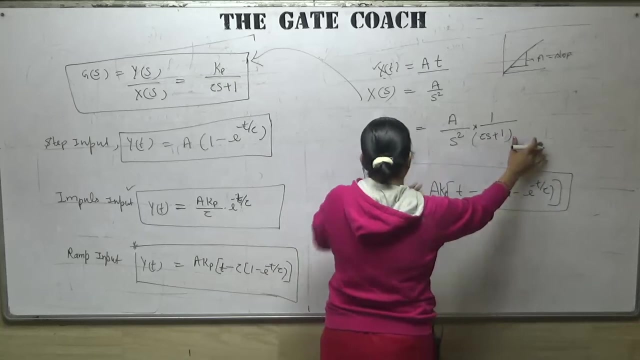 but for the ramp input xt is equals to at and the laplace transform of this xt, xs is equals to a upon s square. substitute this value of xs in your first order transfer function and take the make the pass reflection. take inverse laplace transform, then you will. 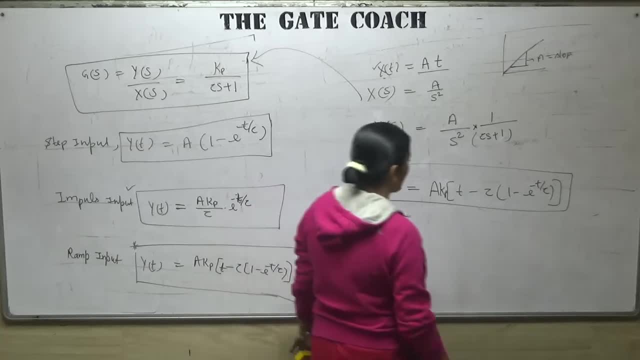 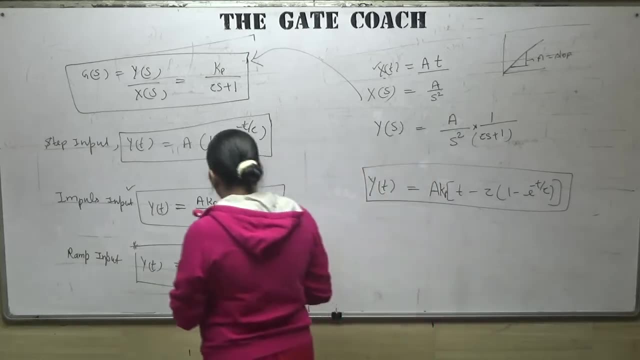 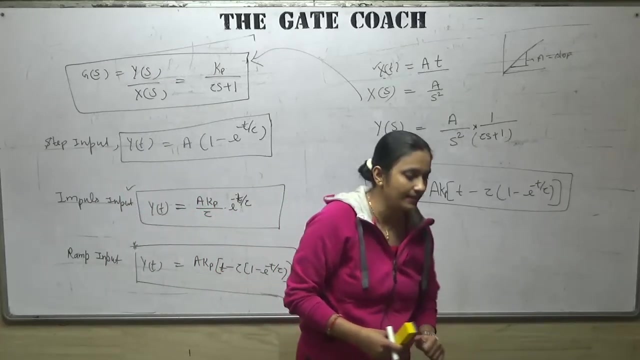 get the response equation. then you will get the response equation. this is the response equation for the ramp input given to the first order system. first order system. it can be your liquid level mixing tank process or your mercury thermometer. few questions of other topics we will discuss. that comes frequently. just first wrote down this. 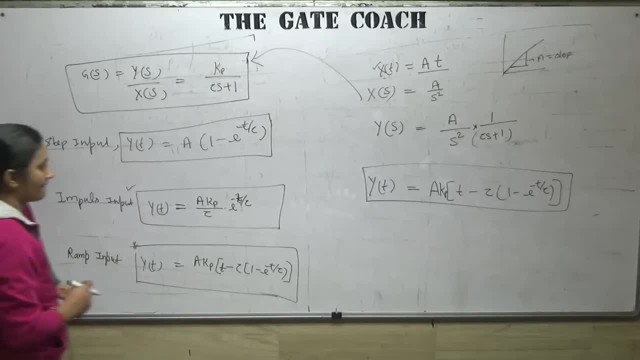 for the different forcing function. we have discussed four, four forcing function, that is, step function, impulse function, ramp function and sinusoidal function. right, what these? how the first order system vary if we are having a process like process of water heating system or either the process of any uh catalytic reaction or reactor. if we are giving 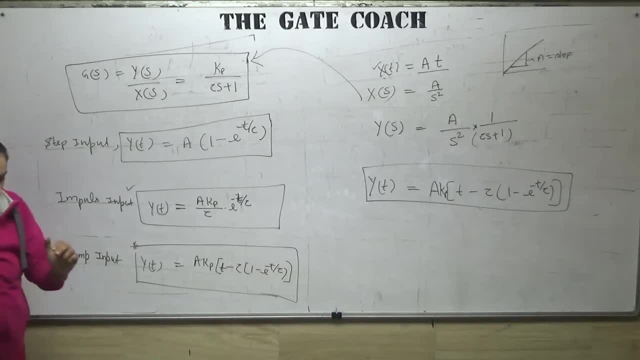 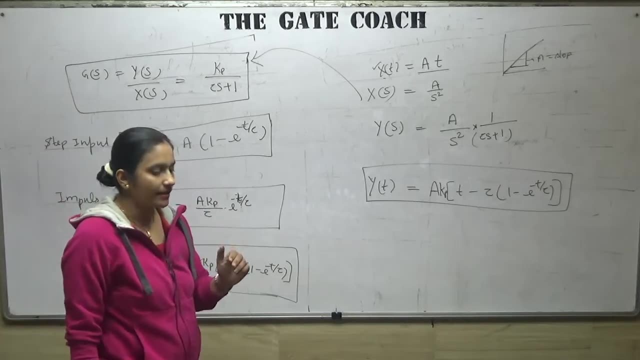 any disturbance in a step manner. how will the response will change if we are giving any disturbance or any forcing function, any change into the process? then how the response will behave for the step input. how will the response will behave for the first order system for a given 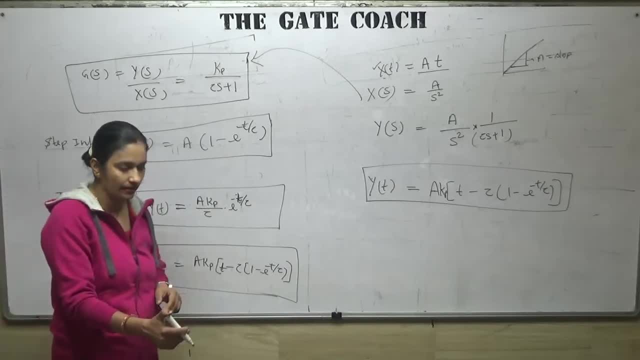 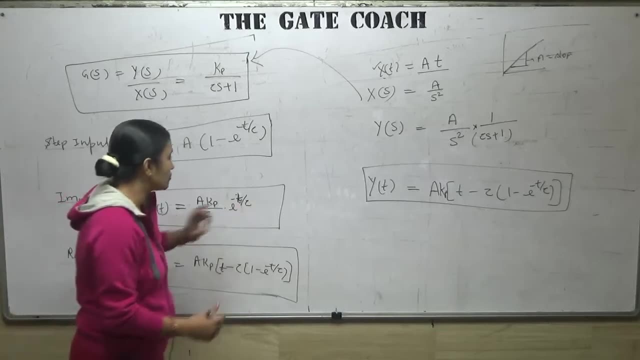 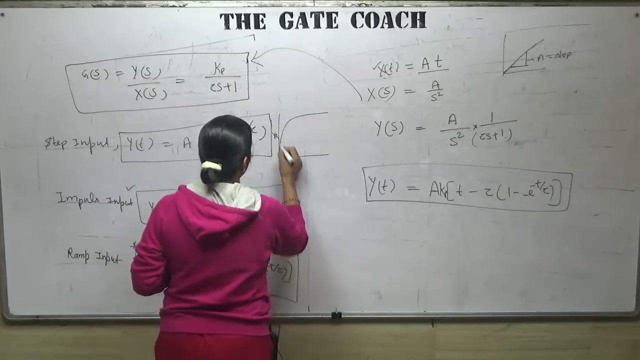 impulse input, like we are if we are injecting anything into the reactor or we are opening a ball and closing the ball, we are getting any impulse input. how does the response will? so? so for the first step- input- we have shown that it will go like this: by t upon t upon tau, and for the impulse, 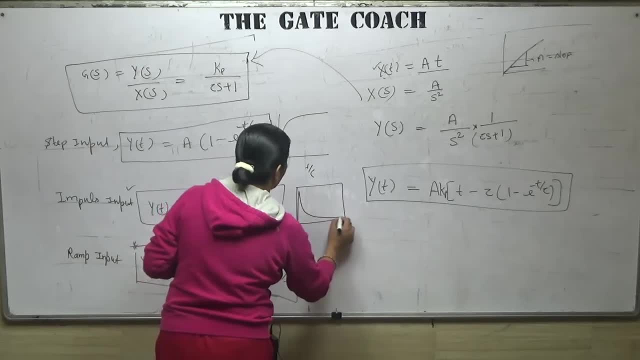 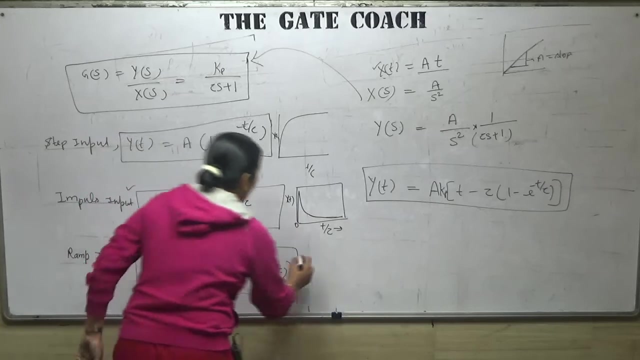 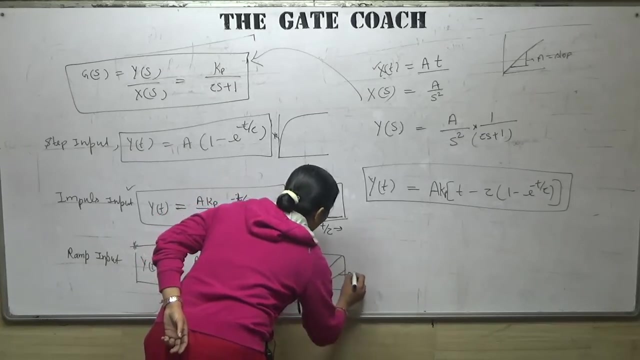 this will go like this means suddenly it will reaches to its higher value and it will decrease exponentially. that is it. it is for the impulse. this one is for the impulse input and the another is ramp input. ramp input is you are giving any input. then it will go like this: this will be the output, this is input and this is some lag. that. 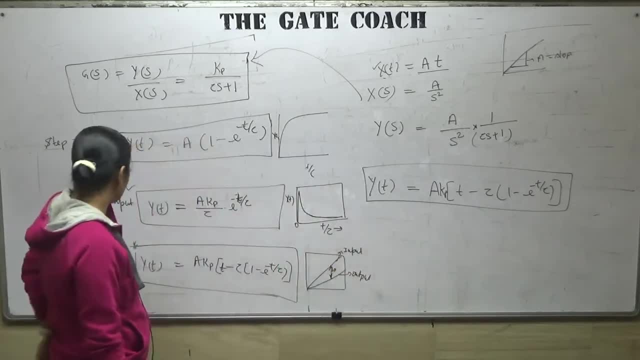 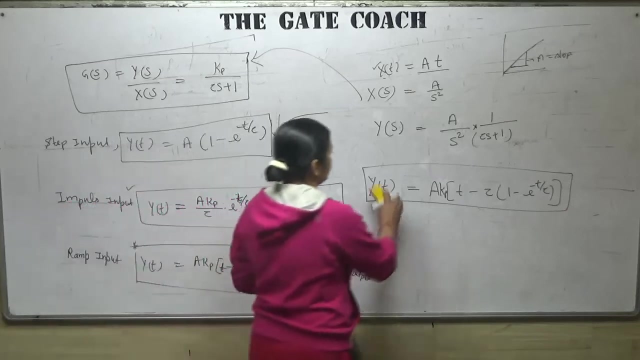 occurs, right? so this one is for the ramp input. now the another forcing function is the sinusoidal forcing function. how does the response will go for the first order system for a given disturbance of sinusoidal input. what is sinusoidal input? x, t is equals to a sine omega t. 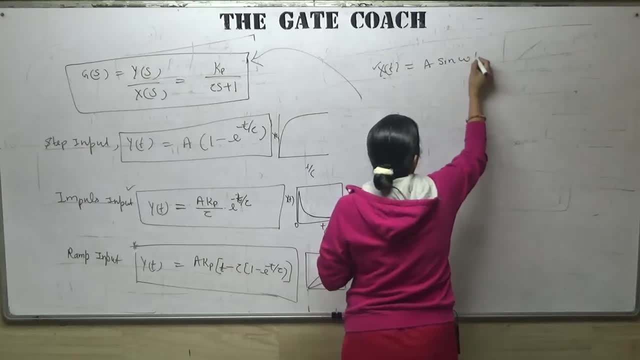 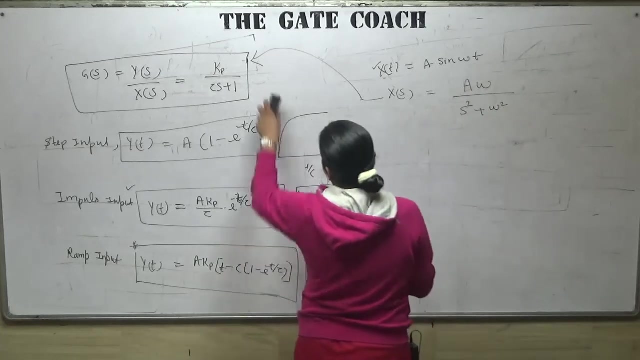 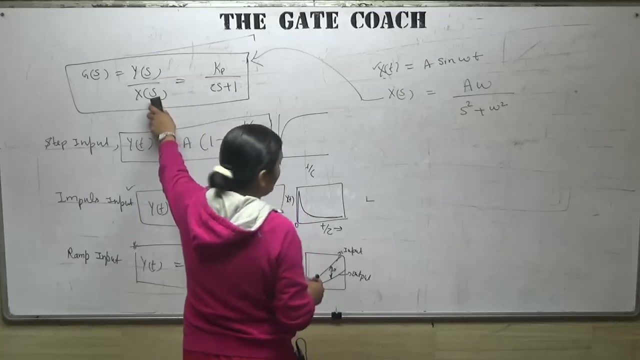 x t is equals to a sine omega t, and what is xs for this is a omega upon s square plus omega square right. when you substitute this value in your first order system, gs is equals to ys upon xs is equals to kp on tau s plus one like: put a value of xs here right, you will get function. ys is n. 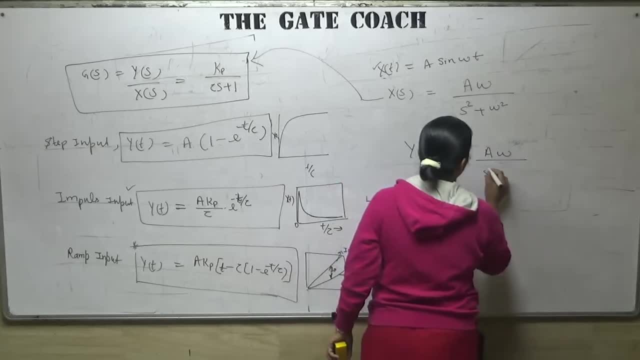 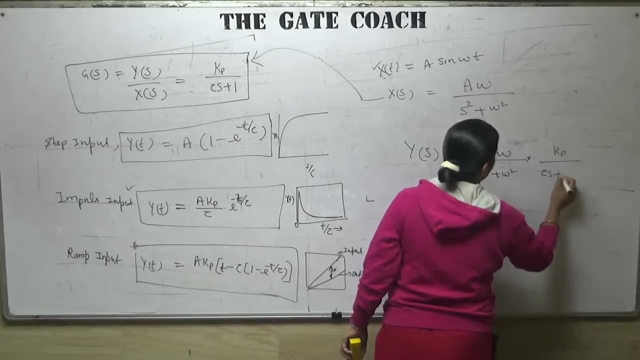 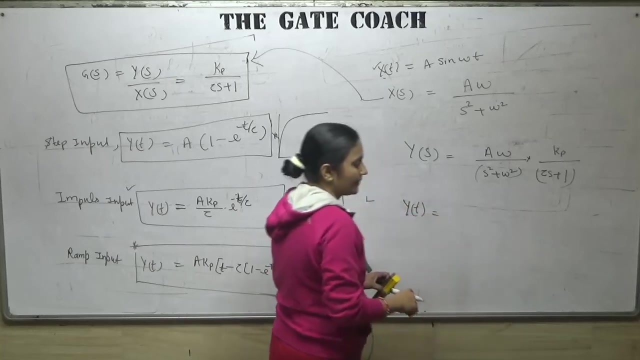 variable: a omega upon s square plus omega square into kp upon tau 8 plus 1, right? so this is what you will get for getting the response. you have to calculate the by ''t''. how you get the by''t' if you are, if you want to convert your equation, 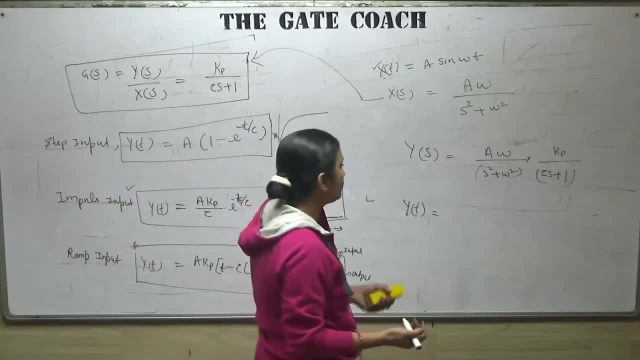 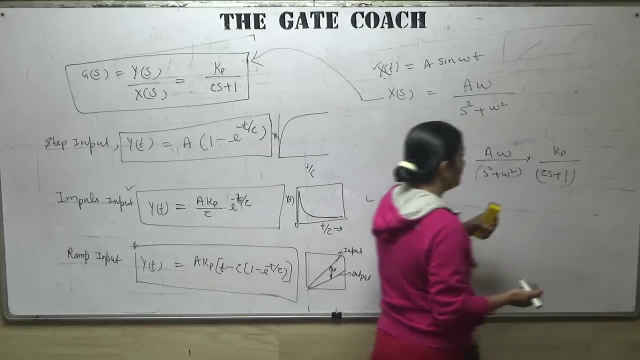 into time domain. you have to take inverse nappletealing also. you just use a lymph node network transform. If you have any such kind of equation, you first take the partial fraction, then you take the inverse Laplace transform. then you will get the equation. When you solve this you will get. 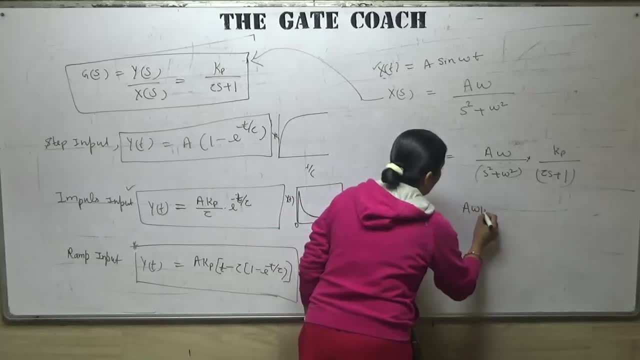 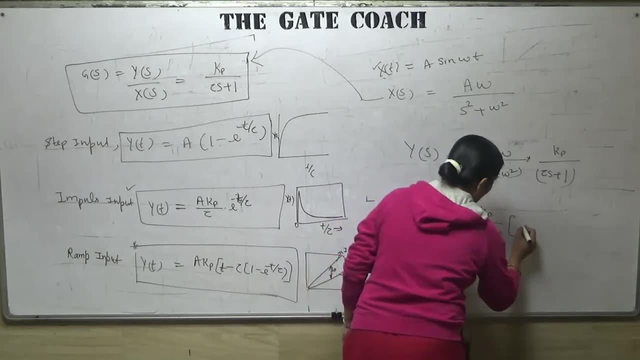 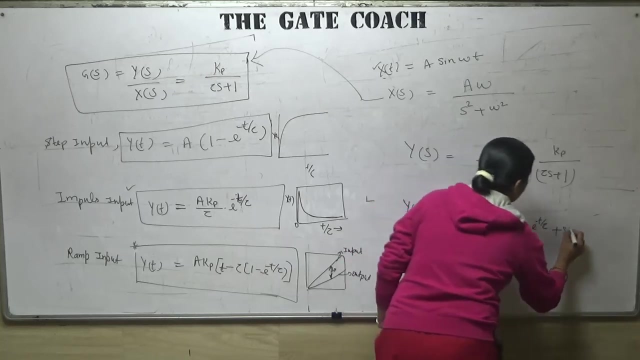 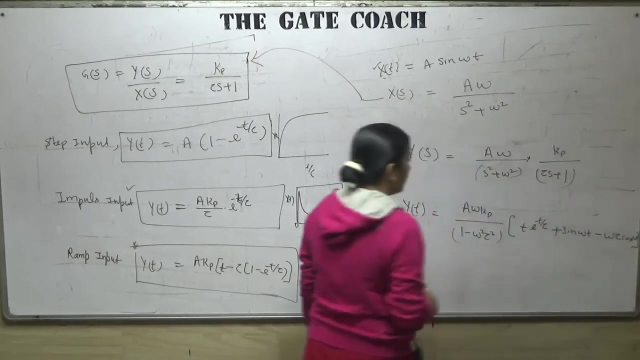 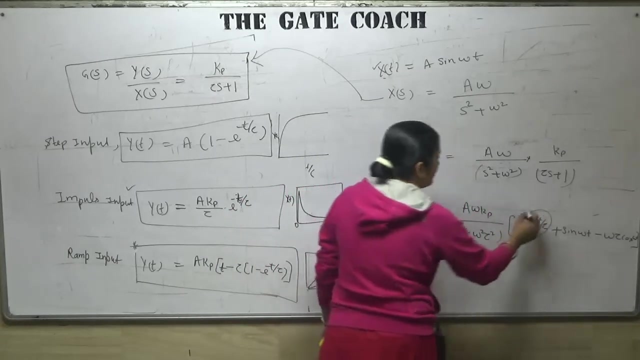 equation like this: a omega kp upon 1 minus omega square tau, square into t, into e, to the power minus t upon tau, plus sine omega t minus omega tau cos omega t. For the simplicity, you will simplify this equation by substituting, by assuming, at any finite time this term will be: 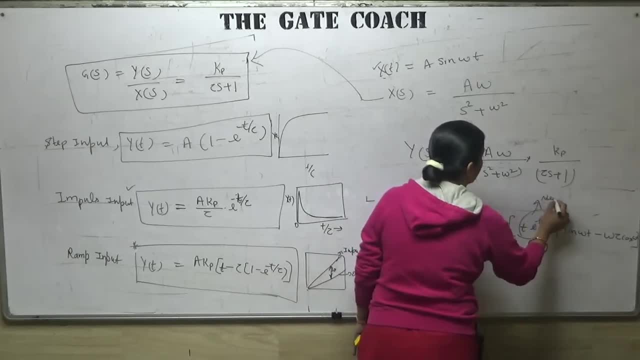 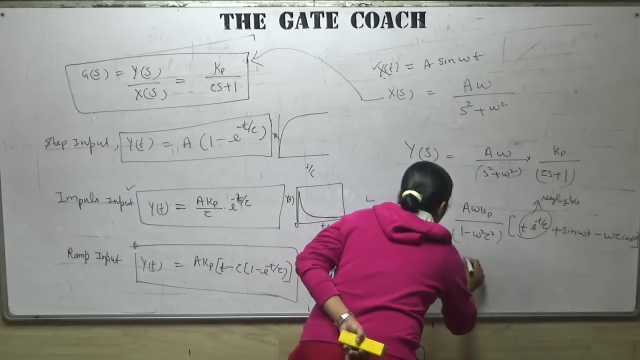 negligible as compared to two other terms. This is negligible And, assuming this, convert this equation in terms of t to the power minus t upon tau plus sine omega t minus omega tau cos omega t. The final terms of this equation will come: a omega kp upon square root of 1 minus omega square. 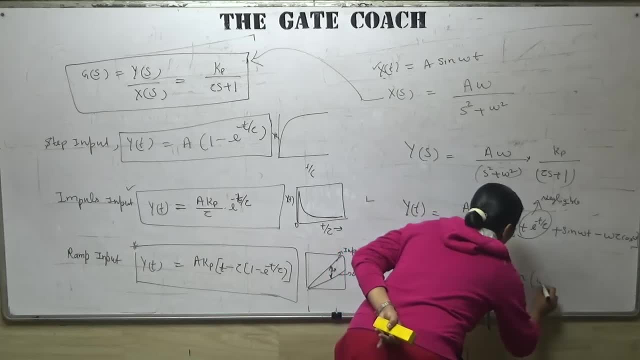 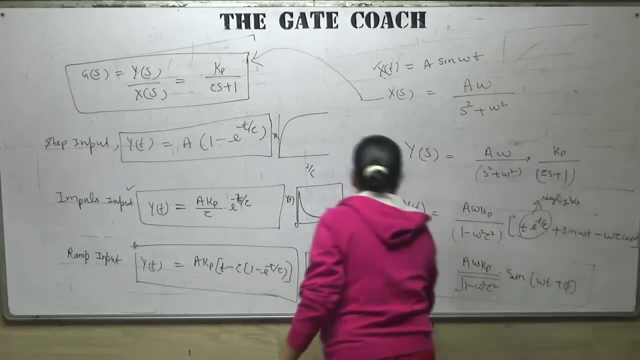 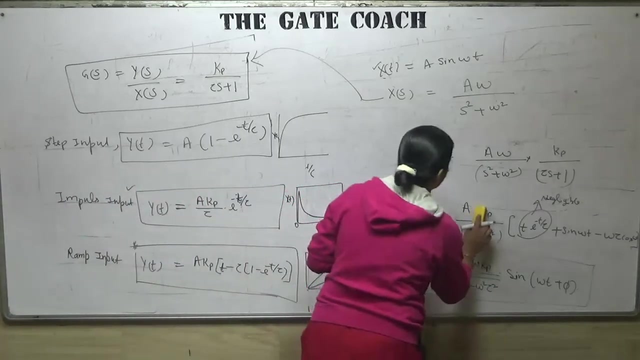 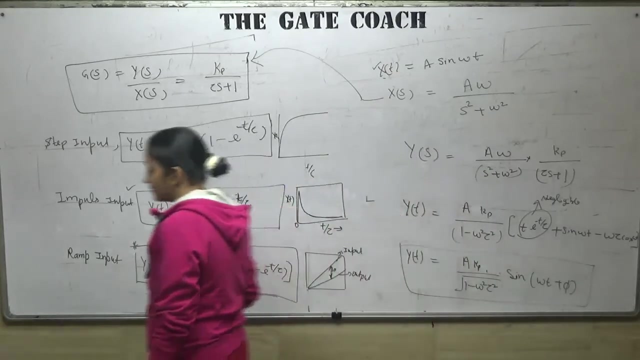 tau square into sine of omega tau plus 5.. So this is the final equation: a omega kp upon a kp, not omega here. in this equation, Yes, omega is not there, Only kp is there. Yes, a kp upon 1 minus. 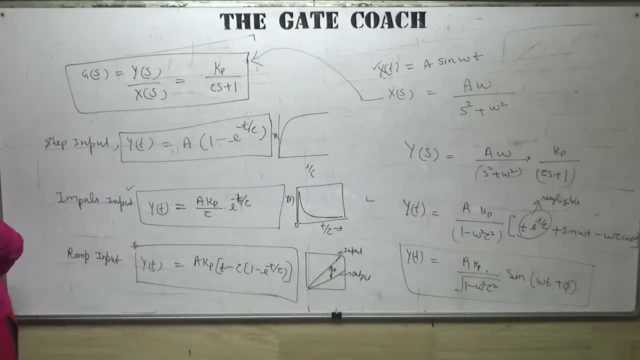 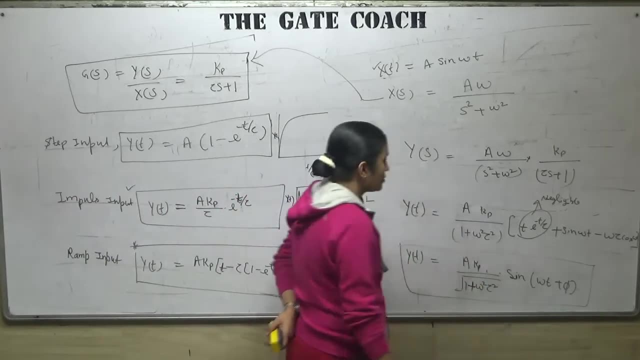 a square root of 1 minus a kp upon 1 plus. Sorry, it is 1 plus. So this is the final equation: a kp upon 1 plus omega square, tau, square. So it becomes a kp upon square root of 1 plus. 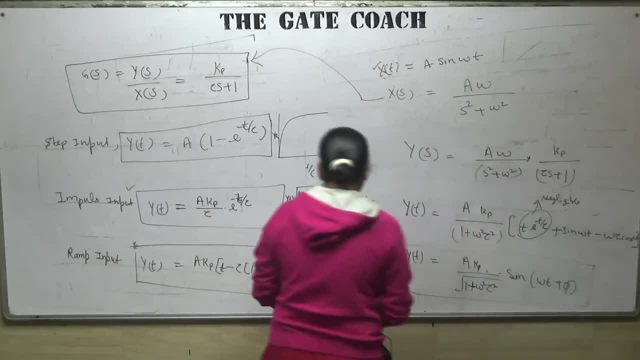 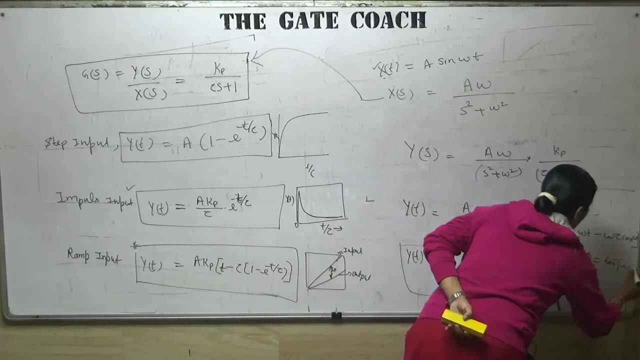 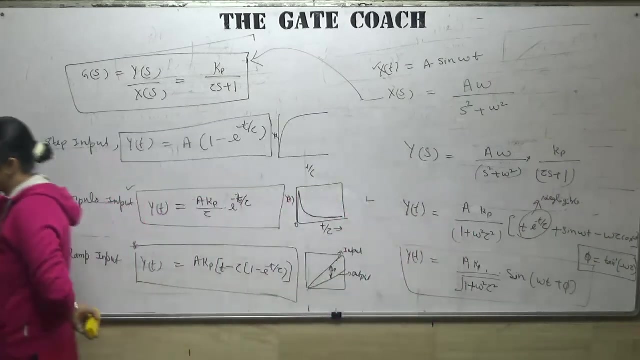 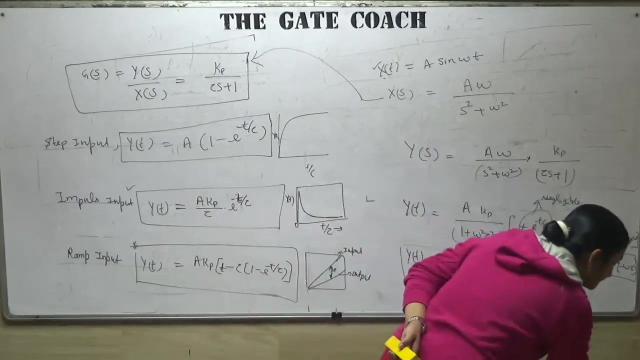 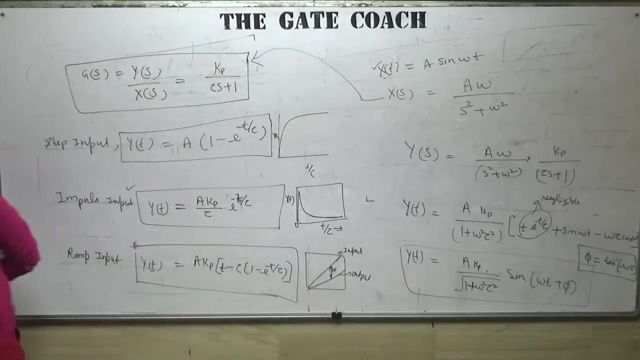 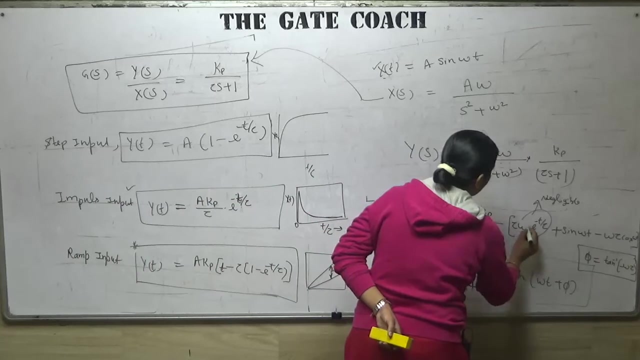 omega square tau square into sine of omega t plus 5, where 5 is equals to tan, inverse of minus omega tau. This is the value of 5.. This is the biotic for your sinusoidal input. How this term becomes negligible. Right, Because this term, this is sorry. tau, omega, This. 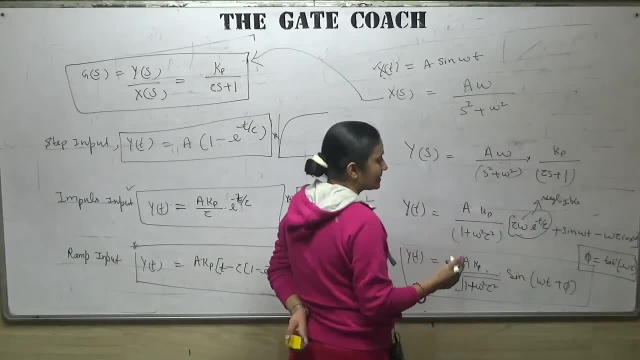 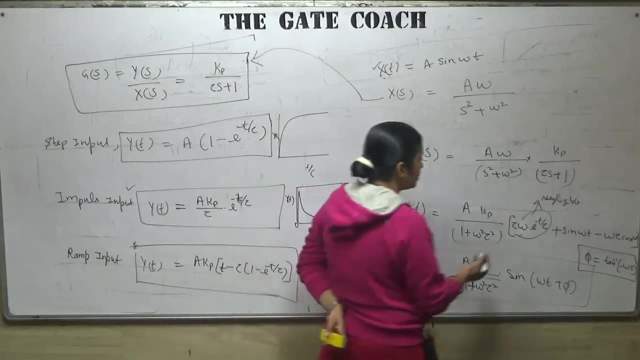 term becomes negligible because at any particular time, as time increases, we are taking a time increases means at any finite time. So this is the biotic for your sinusoidal input. So at any infinite time, or any infinite time, the value of e to the power minus infinity. 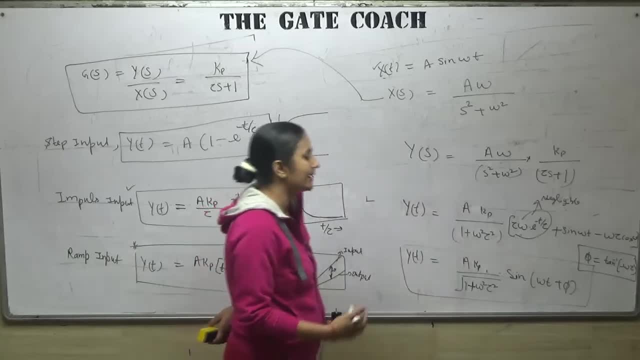 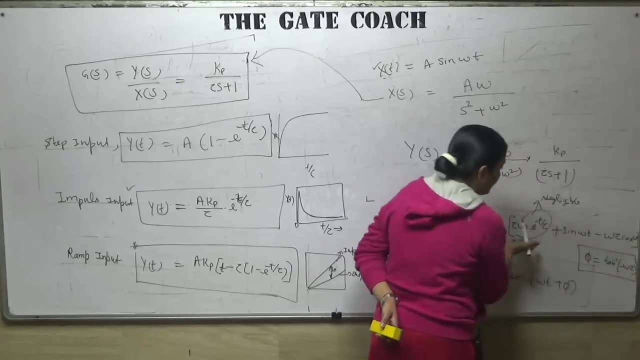 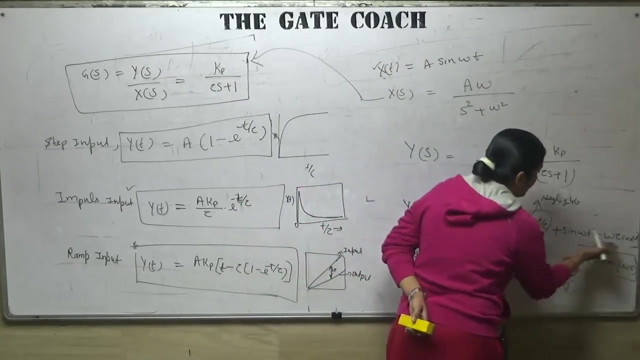 is 0. Or we are taking it as negligible means. as time increases, this is very less value as compared to in these values. So we are neglecting this value Right. And after neglecting this value, we are converting this into the form of sine a, into sine a, sine b minus cos. 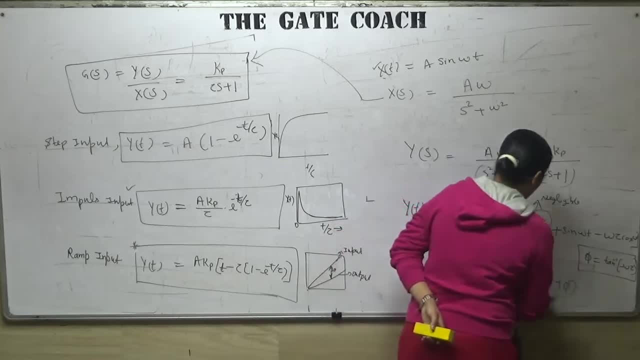 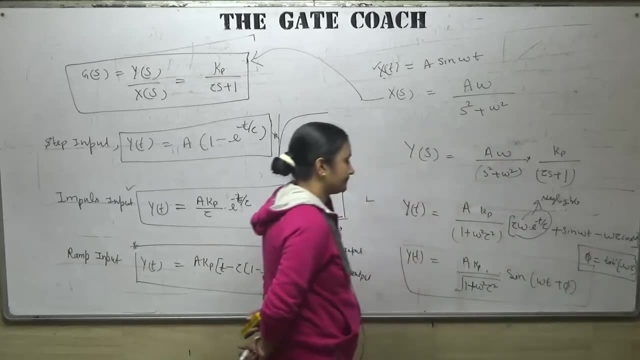 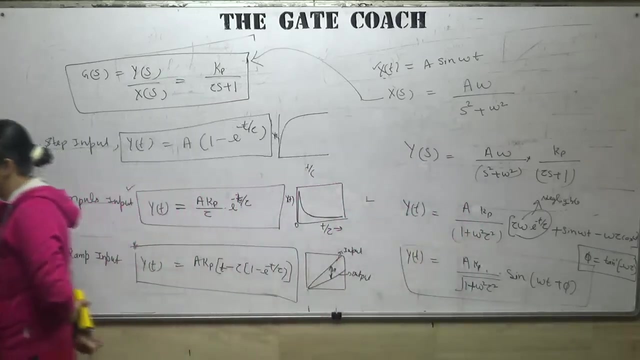 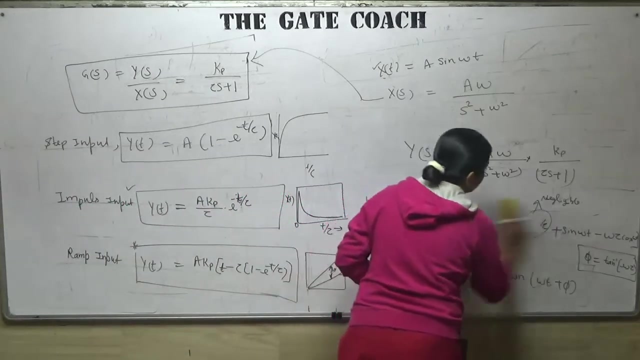 a cos b, like this, And you will get the value of phi as the final in Sine of omega t plus phi, And phi is tan inverse of minus omega tau. Yes, Do you get your point? Yes, So here how we obtain this: In this, a is the amplitude. 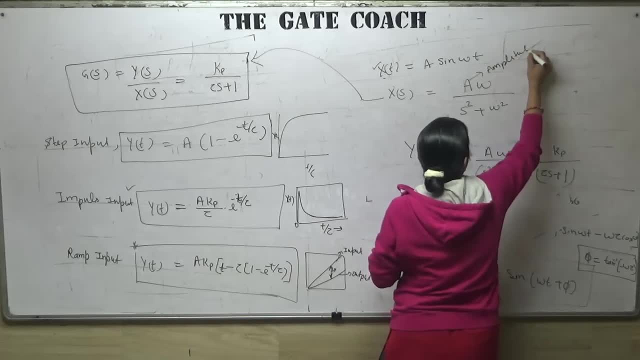 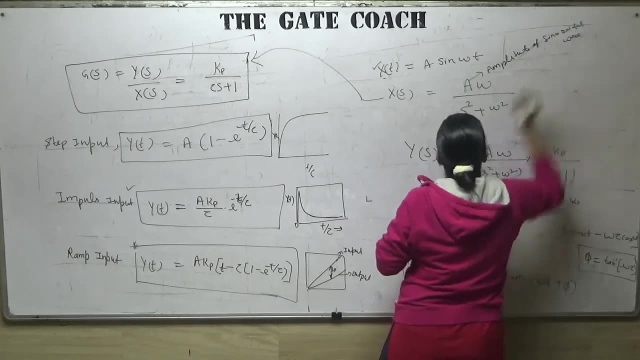 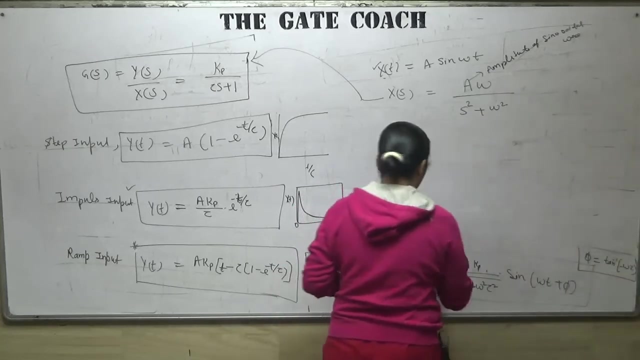 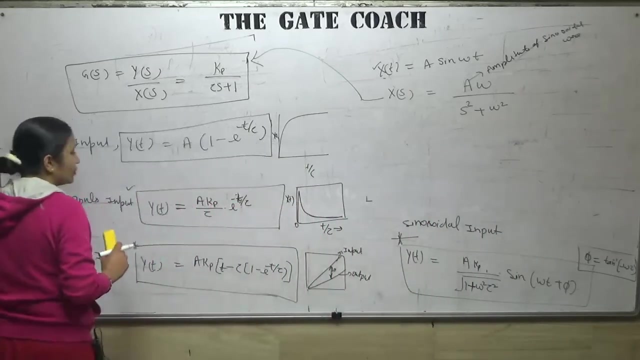 A amplitude of sinusoidal wave. Amplitude of sinusoidal wave. Write down: this is the formula for sinusoidal input for the first order system. Right, All these are the you different forcing function given to the first order system for the snap input, the response. 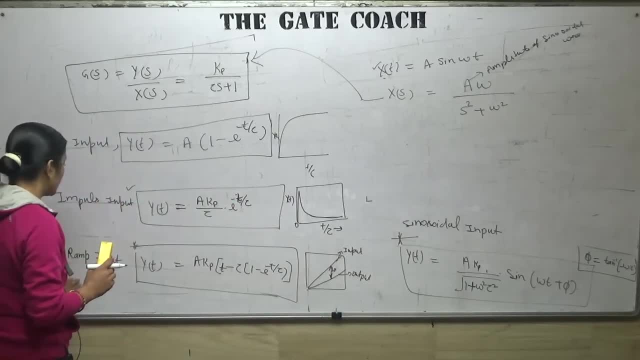 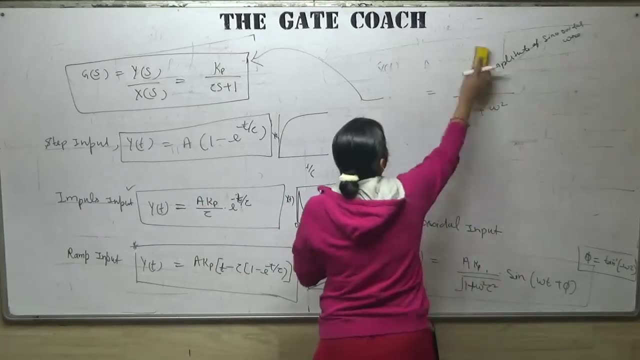 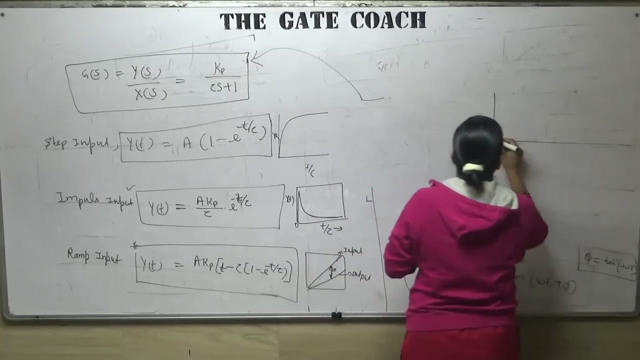 formula is this: for impulse input, the response formula is: for the first order system. for ramp input is this: and for the sinusoidal input, the formula is this: and the output curve or the characteristic for the sinusoidal wave will go like this: this is the input curve, this one is the input curve, or we can say: this one is the XT and the. 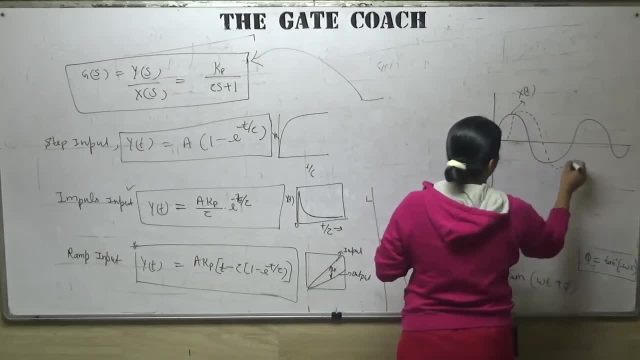 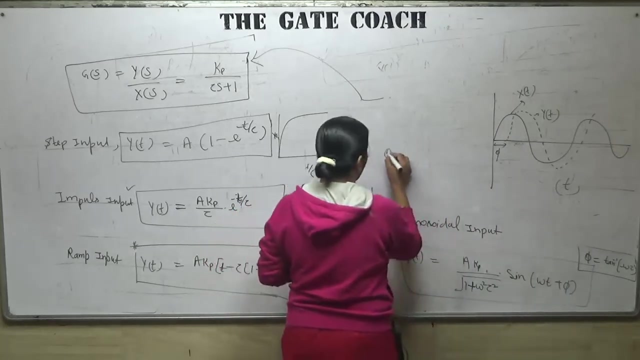 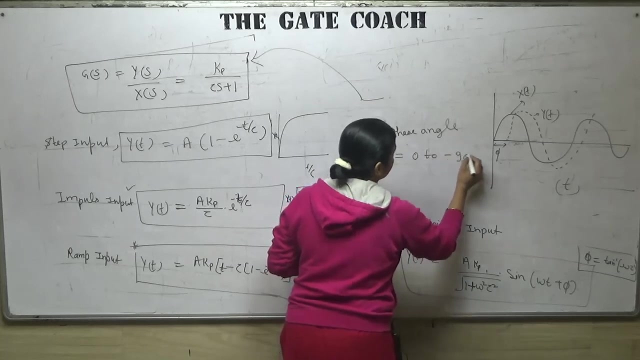 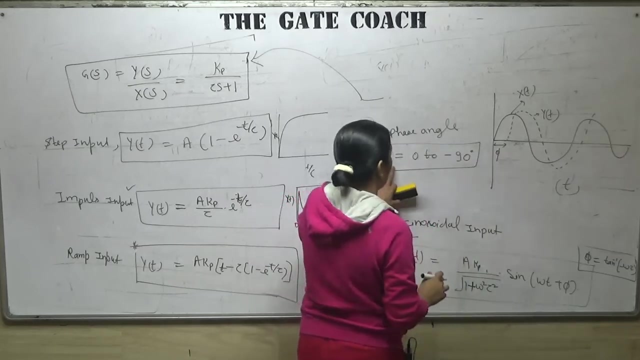 YT will come after some phase lag. phi, that is the YT right. so this is a graph. and phi for the first order system. phi- the phase angle, phase angle: right. so this is the graph. and phi for the first order system. phi- the phase angle. phase angle barises from 0 to minus 90. minus 90 degree. the phase angle for first order system is barises. 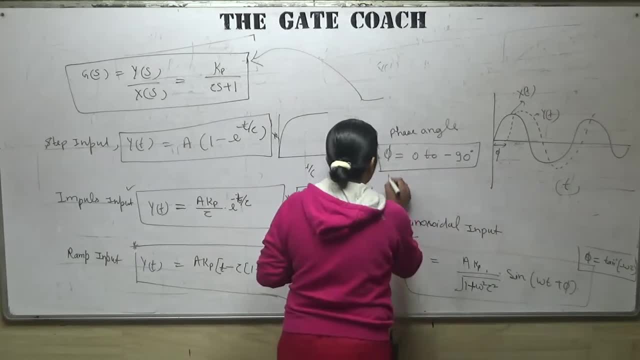 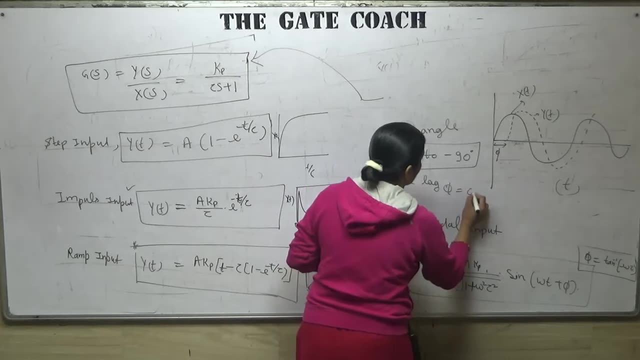 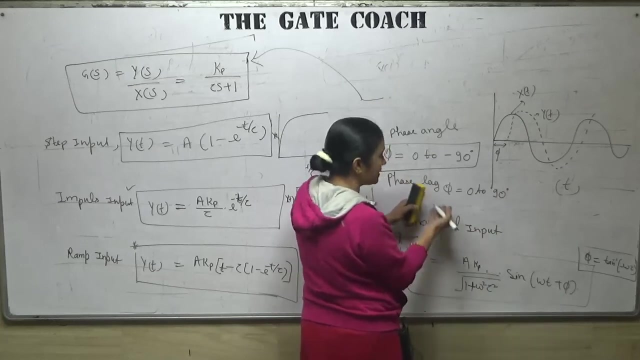 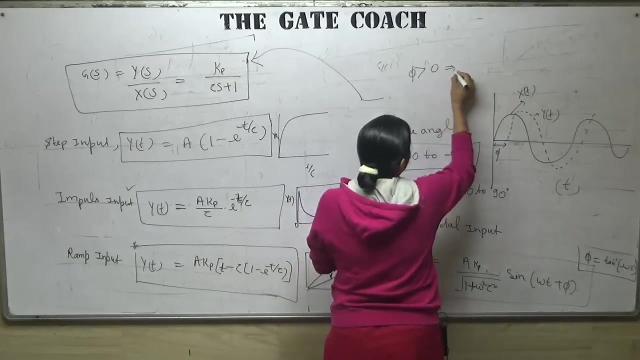 from 0 to minus 90. if we are saying phase lag, phase lag means the phi is 0 to 90. lag means behind. behind means it's obvious, it's negative. lag means negative. leads means positive when your phi is greater than 0. greater than 0 means positive, means lead. this is called phase lead or lead. 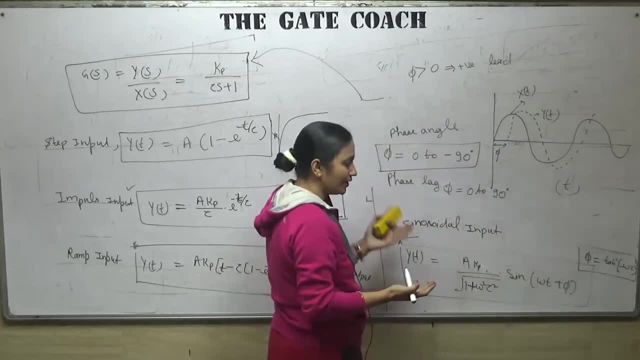 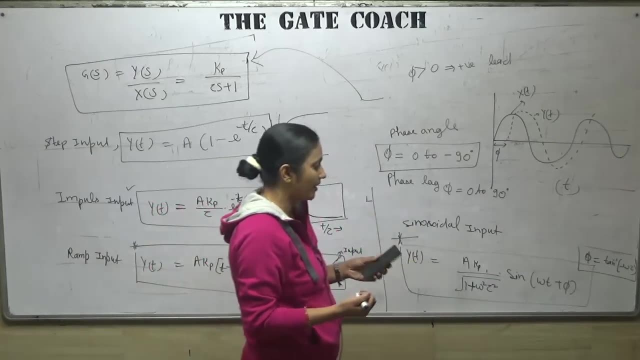 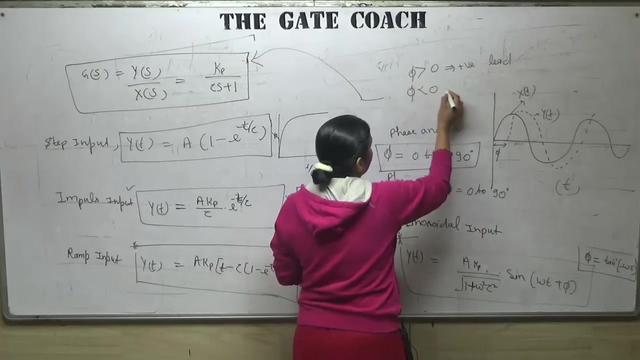 process. lead process means your output is leading to the input. that is practically impossible. output cannot lead to the input. always we first given the input, then it will followed by the output. so phi is always be less than zero and it is negative. when it is negative, then we say: that is. 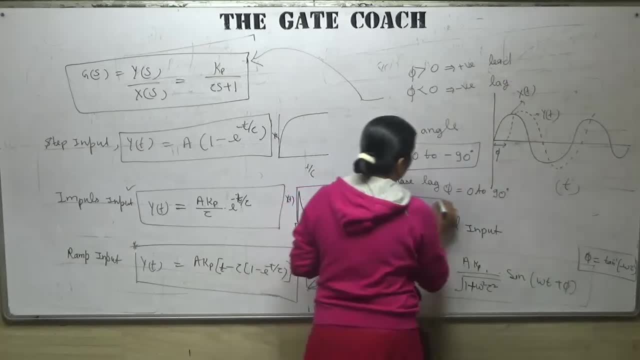 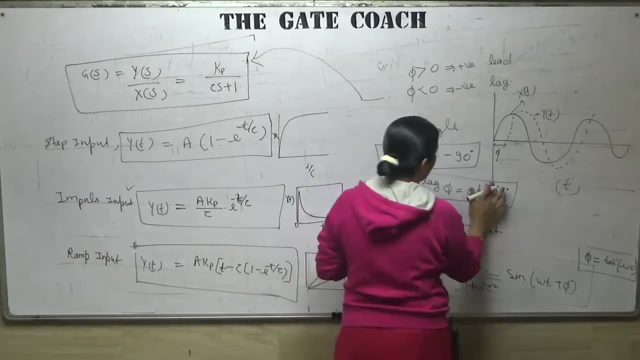 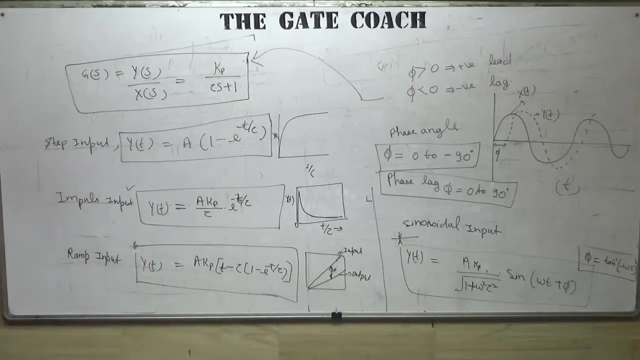 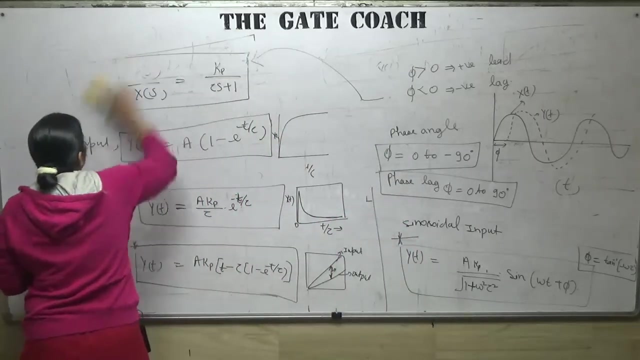 a phase lag, right. so if we are saying phase lag, then we say it is 0 to 90. if we are saying phase angle, then it is 0 to minus 90. for the first order system. yes, note down this. so, okay, i am placing this one more thing into the sinusoidal input. this is the last topic. 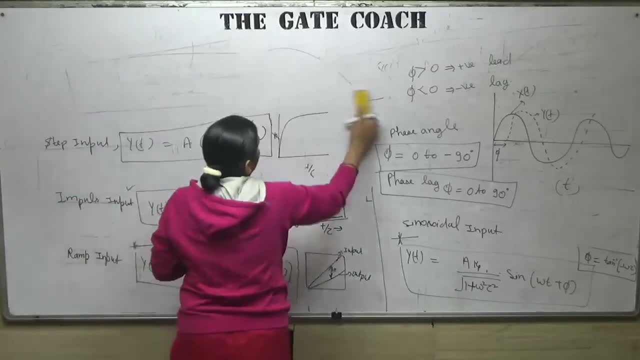 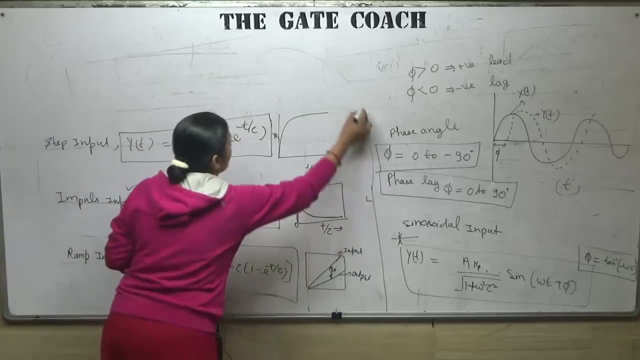 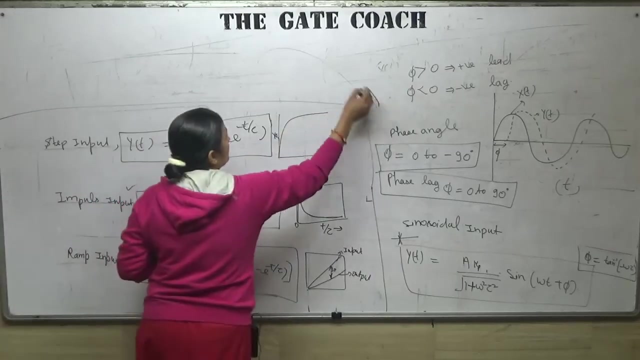 the remaining topic we will discuss tomorrow. so one more thing. i am placing this, one more thing into the sinusoidal input. this is the last topic. what is amplitude, amplitude ratio? we will. if we are talking about the amplitude ratio, we are talking about the sinusoidal step input, amplitude ratio. 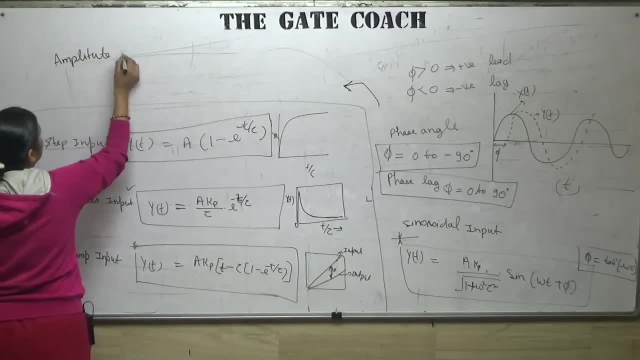 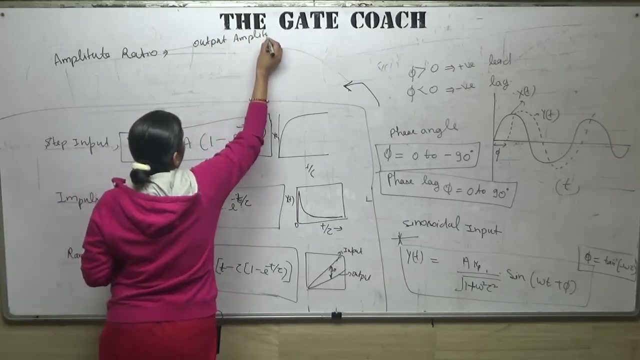 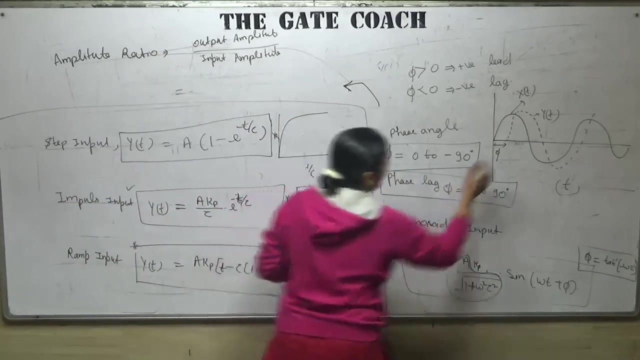 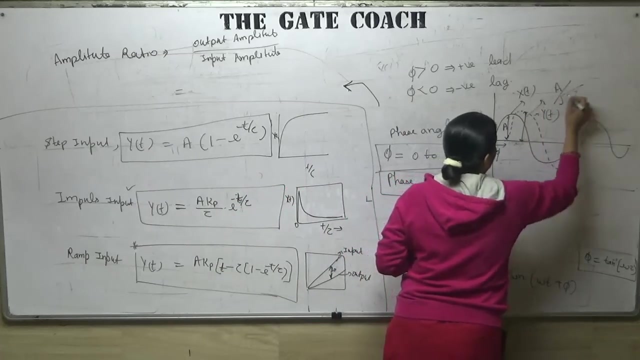 what is amplitude ratio? amplitude ratio is defined as output amplitude to the input amplitude. all good, amplitude to the input amplitude. that is nothing but output amplitude. here our is this output amplitude: the input amplitude is a and the output amplitude here is a coupon, a square root of 1 plus omega, square and chapter. so what is the value of amplitude ratio is? 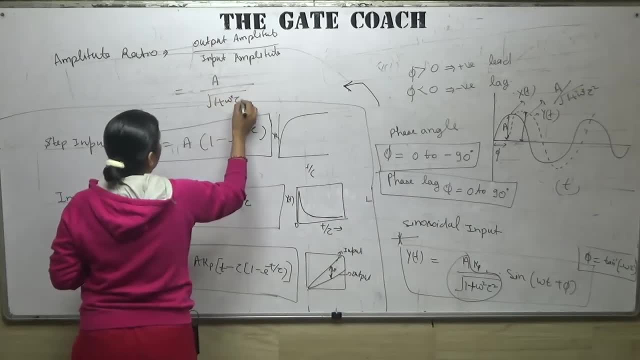 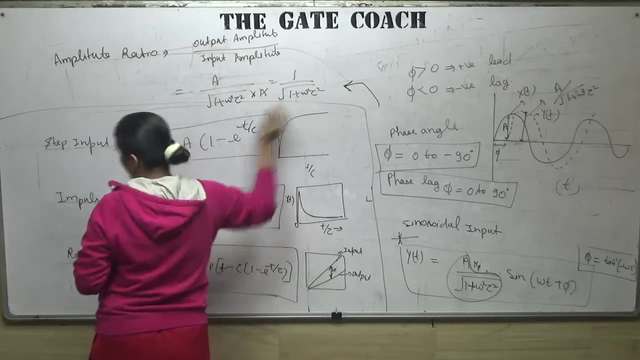 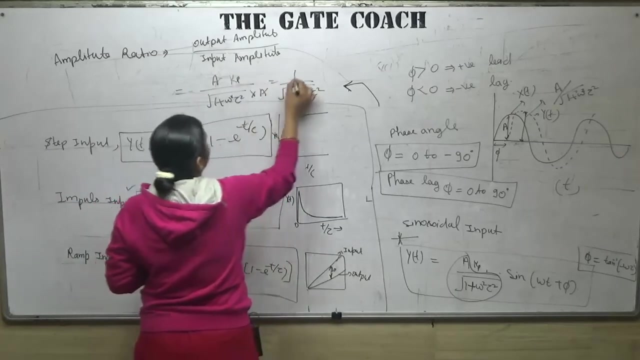 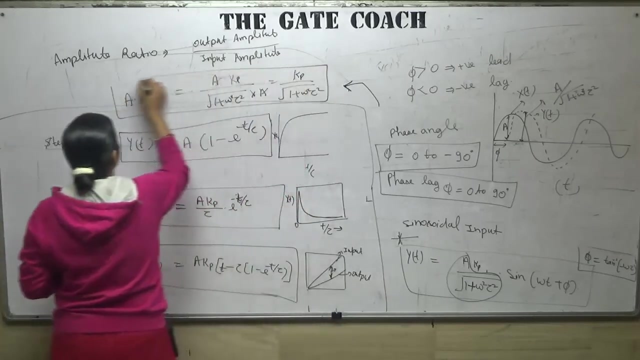 a upon square root of 1 plus omega square, tau square to a. a, a get cancel it come 1 upon square root of 1 plus omega square square. that is your amplitude ratio. if you the kc is there, you can write it as kp. this is the amplitude ratio. things to remember in sinusoidal wave is your response. 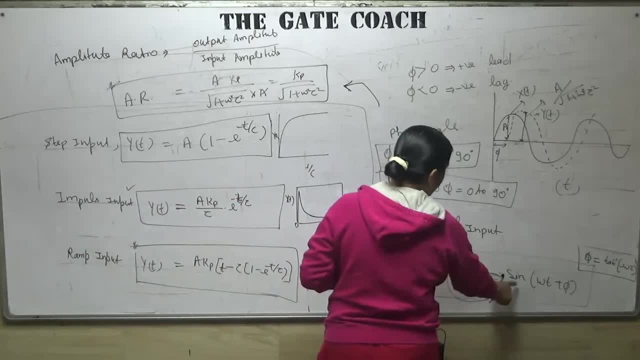 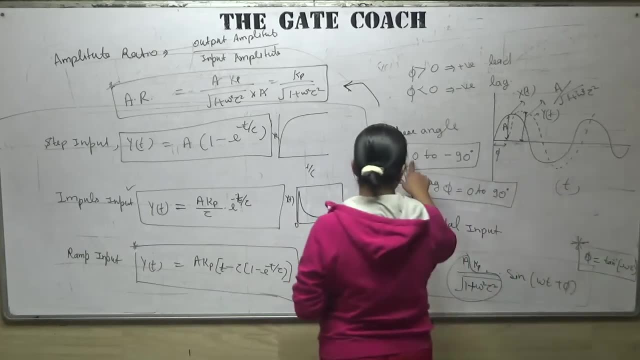 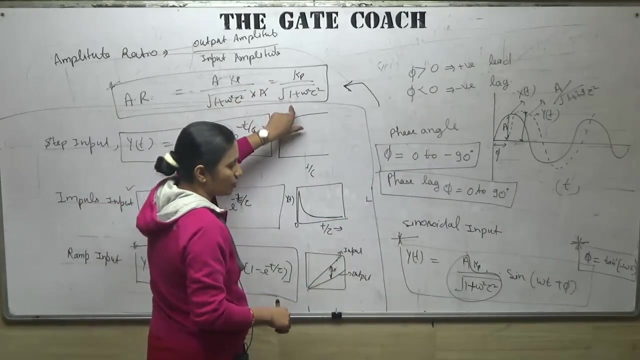 equation like a kp upon square root of 1 plus omega square pi square, sine omega t plus 5 and the phase angle phi is tan inverse minus omega tau that varies from 0 to minus 90 angle and its amplitude ratio is kp upon square root of 1 plus omega square tau square. is there any doubt from? 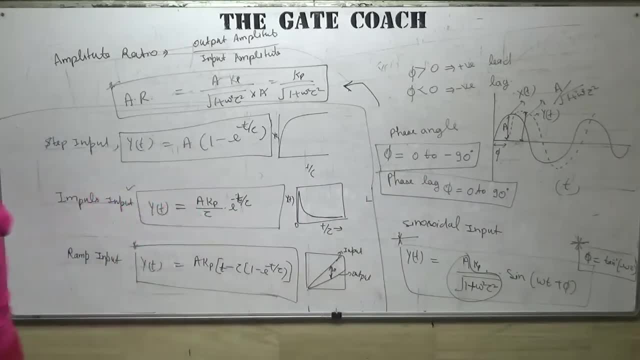 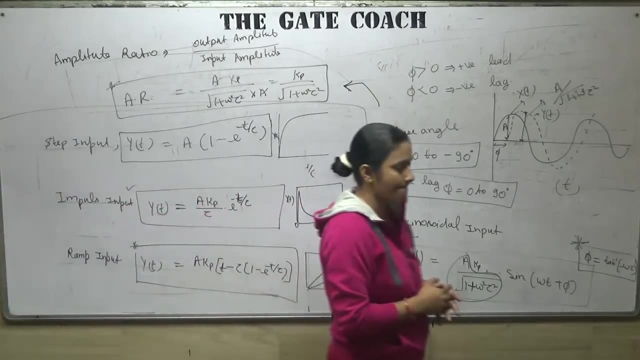 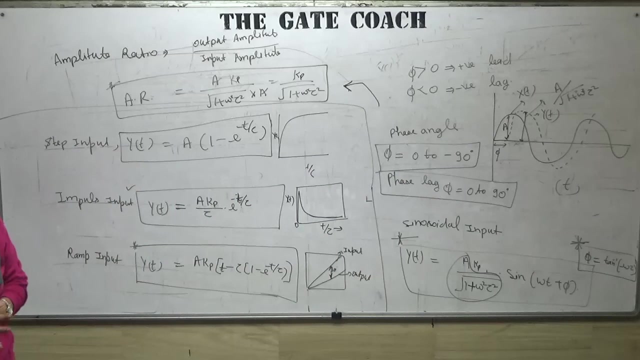 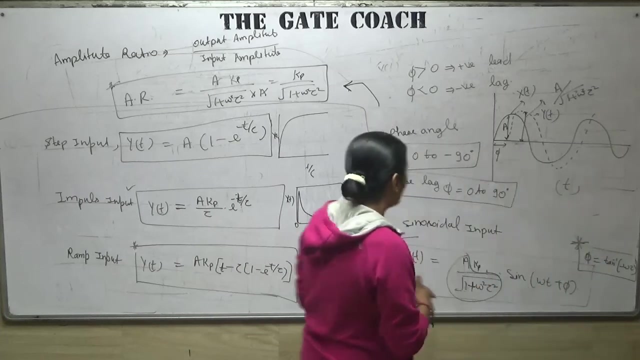 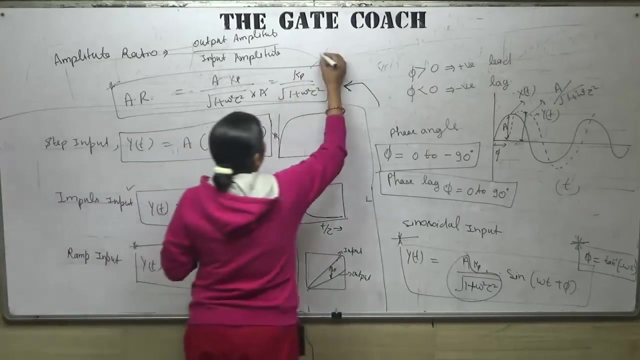 uh, the starting to till this topic. we will conclude the class here. yes, is there any doubt? range of the amplitude ratio. amplitude ratio will always be less than 1. it will always be amplitude ratio. good question. amplitude ratio will always be less than 1. it cannot be greater than 1, if your 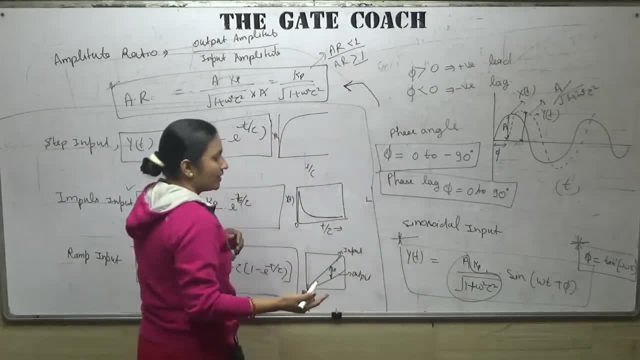 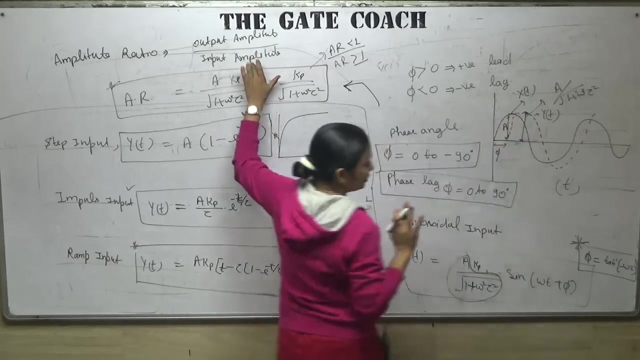 amplitude ratio is shown. greater than 1 may means the system is not as stable. greater than 1 means what does it indicate? what is amplitude ratio? output amplitude to the input amplitude. output amplitude cannot be greater than your input amplitude- or graph will be so, i guess- but output amplitude cannot be greater than your input. 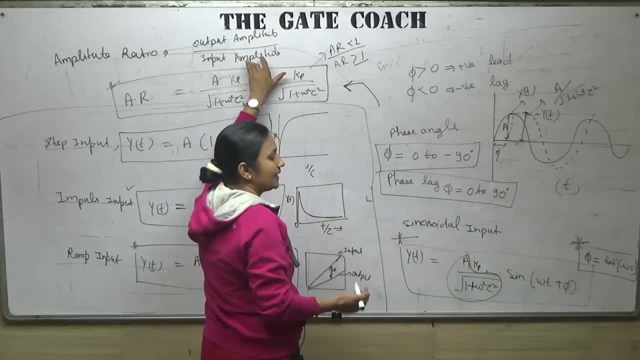 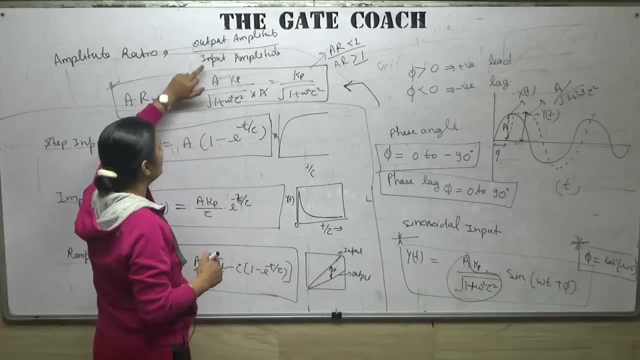 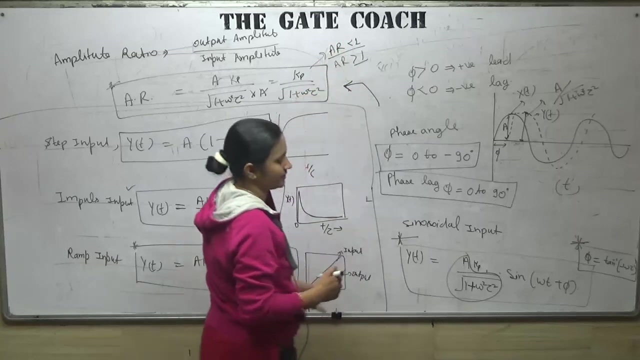 amplitude. if your output is greater than input means it is a leading process, right, right, so it is. uh, the output is less as compared to the input, so this will be always less than 1 for the stable system. if amplitude ratio is greater than 1, it is an unstable system. yes, it is clear to you. 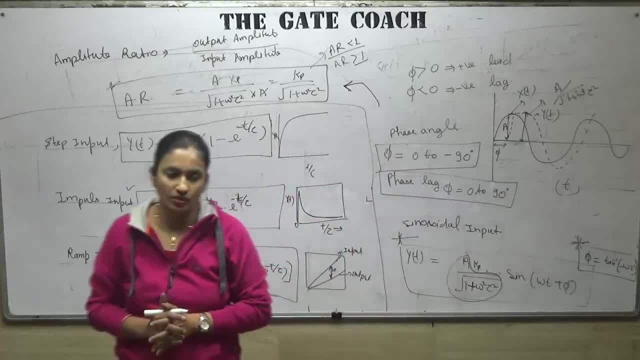 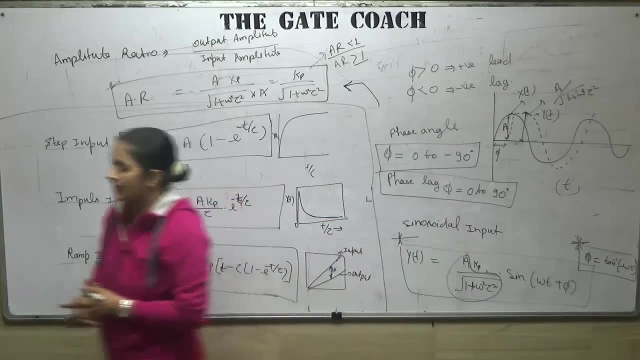 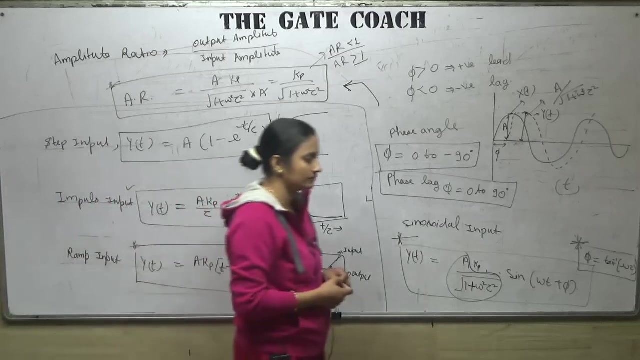 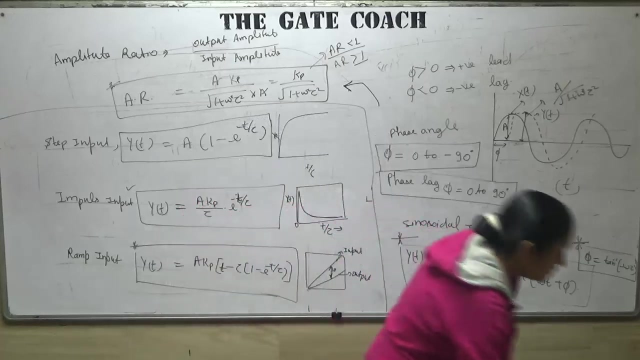 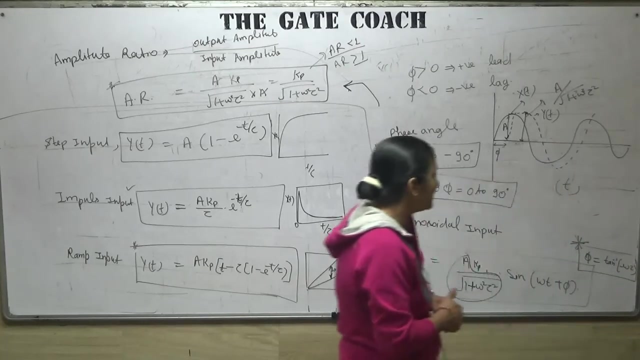 this can be asked. the value of amplitude ratio bearizes for the first order system for a stable condition, that is, amplitude ratio should be less than 1 for this stable condition. yes, okay, should we leave the class now or is there any doubt? yes, okay, thank you, glass. repeat dead root example. repeated root examples means not getting the 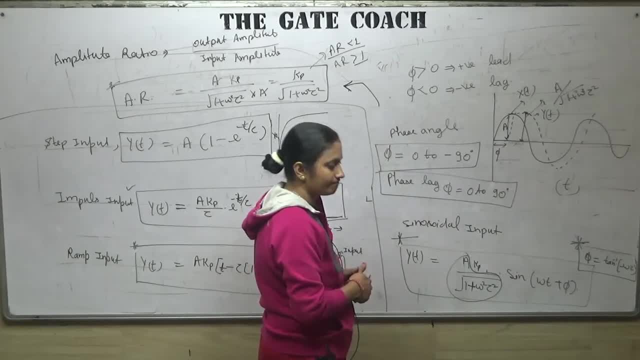 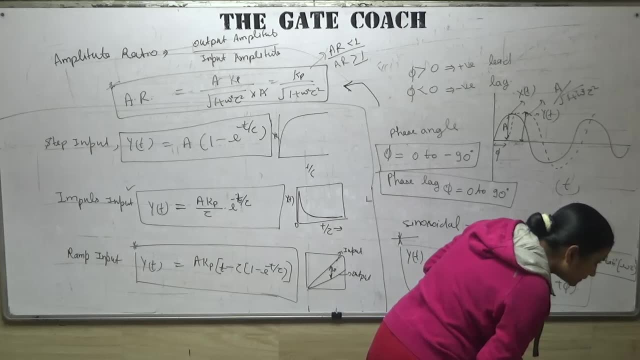 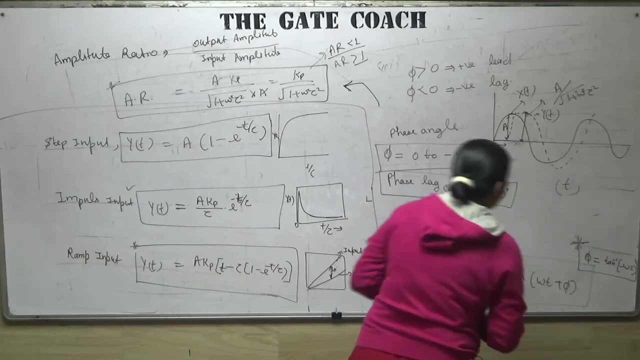 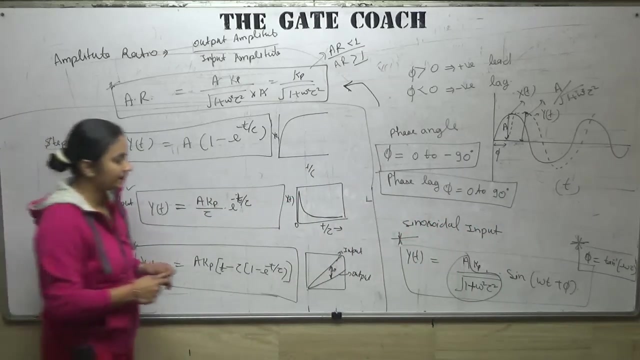 question. I am please explain phase angle in detail. phase angle: phase angle is 5. that is denoted by 10 inverse omega tau. how does this come? I have not. I have not solved whole derivation because it will take time as your equation comes, like we have. 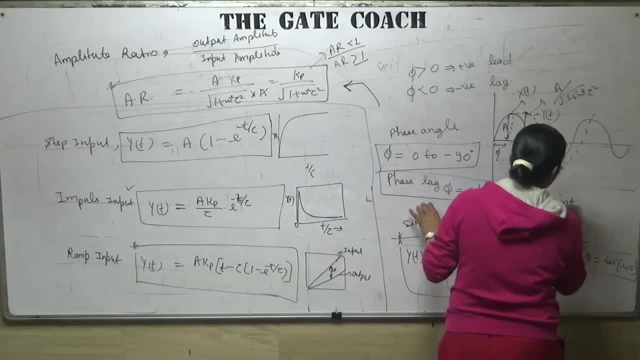 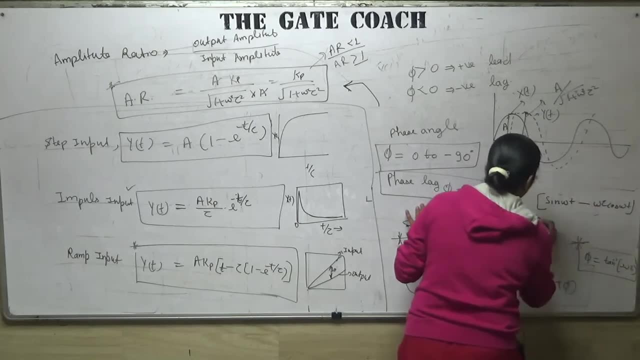 neglected that it will come become the remaining term: become sine omega t minus omega tau cos omega t. in that case we assume that like r sine omega t is r sine omega t is, we are taking it as like not omega t. r sine phi is as 1 and r cos phi is as minus omega tau. right, we substitute these value here, then we: 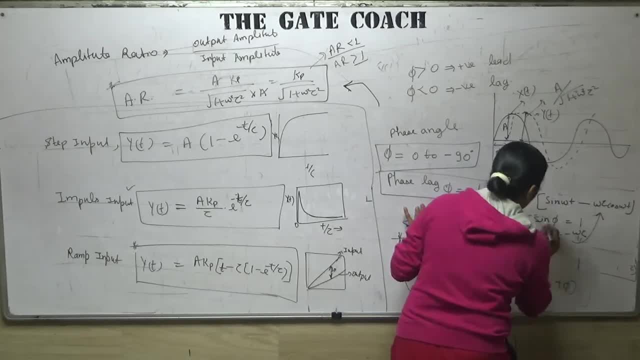 convert it into the value of omega t and we get the value of omega t and we get the value of omega t, but in term of sine of a plus b form, and we get the value of minus. omega tau. phi is equals to minus of 10 inverse omega tau, minus of 10 inverse omega tau. from this right, so from here, this is the value. 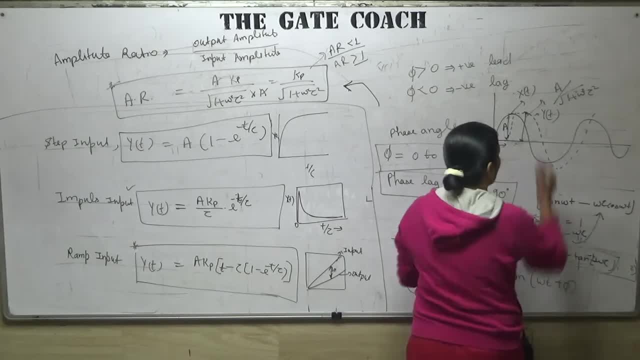 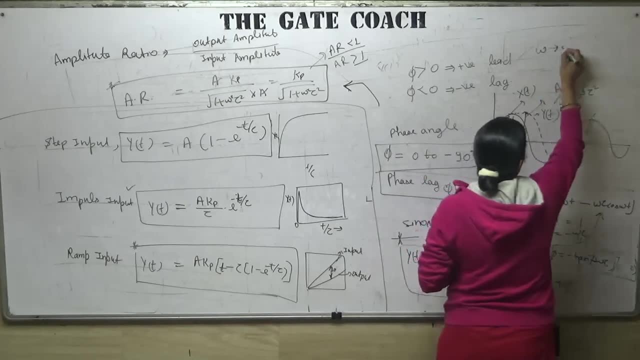 of phi and how it varies from 0 to minus 90. because if you are taking a Bode plot, we will discuss this in detail in Bode plot- that when your phi varies from 0 to infinity, from the equation your value of phi goes from 0 to minus 90. only that. that's where that phase angle. 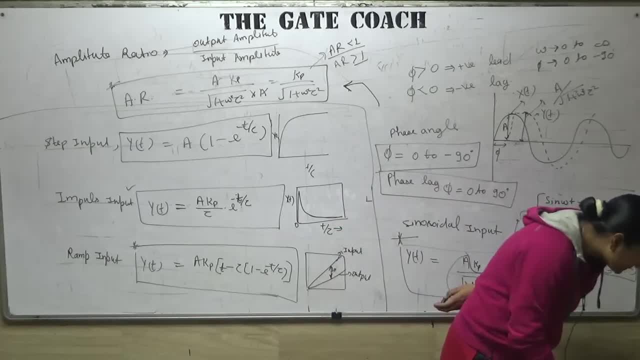 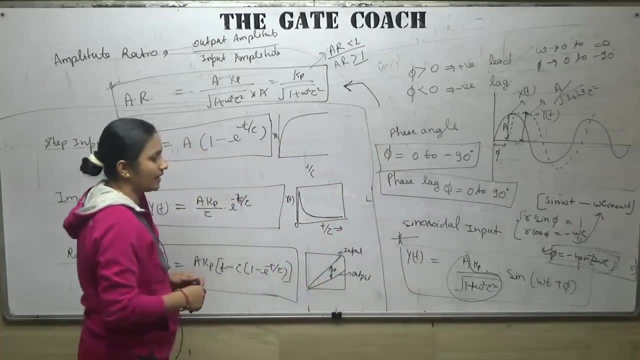 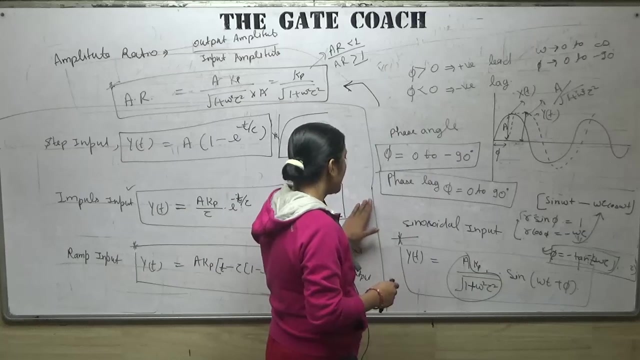 will come inverse Laplace transform. inverse Laplace transform means that is not the repeated. we are not taking the example of that partial fraction. the partial fraction is the other part of that. this is the syllabus, this is your syllabus. that is thus for sinusoidal input. 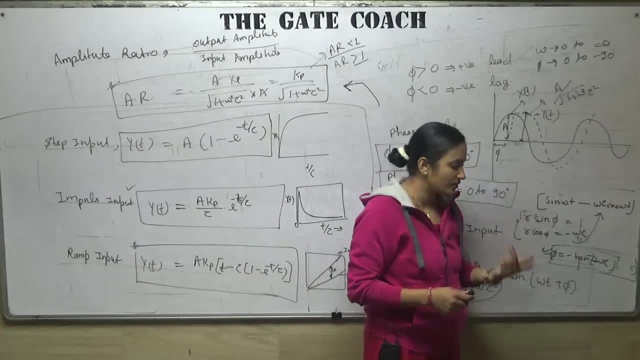 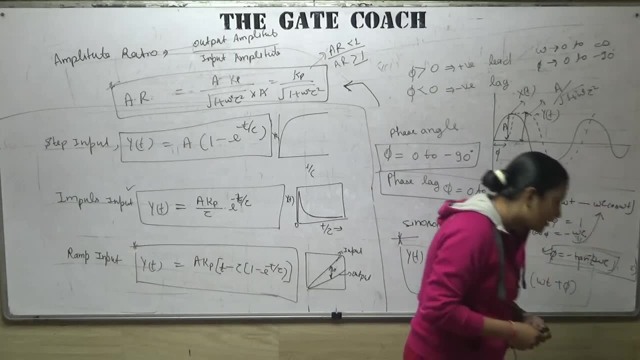 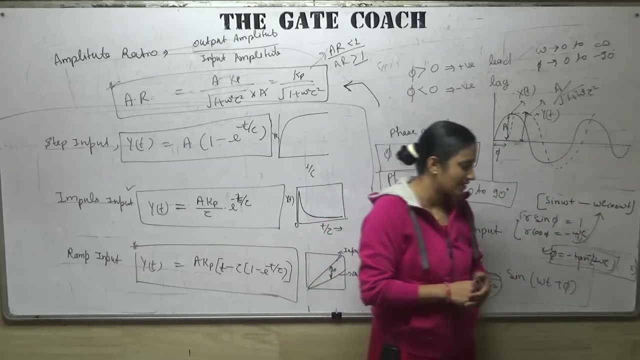 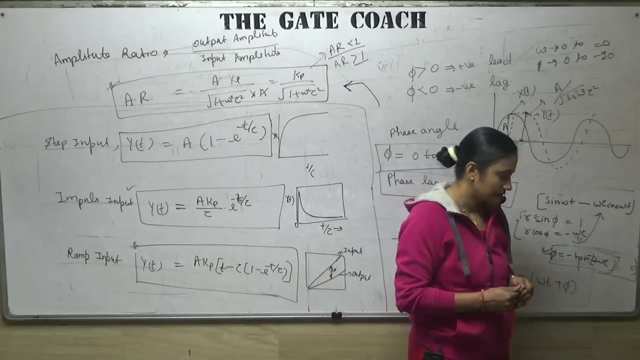 how does your response changes for the first order system in Laplace transform repeated and non-repeated equations? repeated and non-repeated equations means you are saying about the partial fraction repeated roots and non-repeated roots. is it in inverse? Laplace transform the repeated and non-repeated equation? repeated and non-repeated. 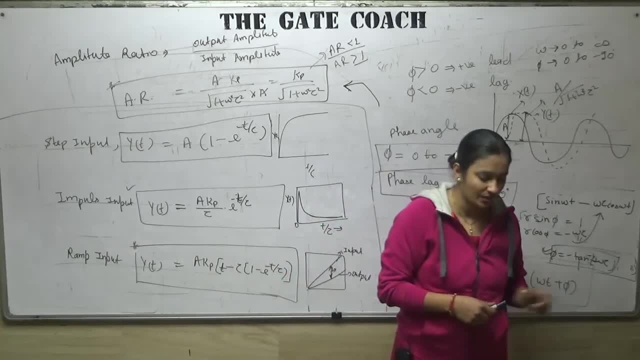 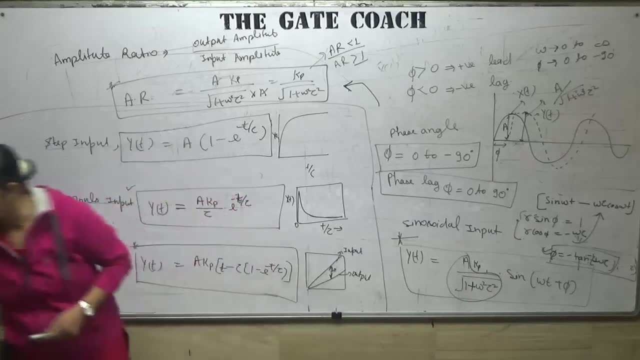 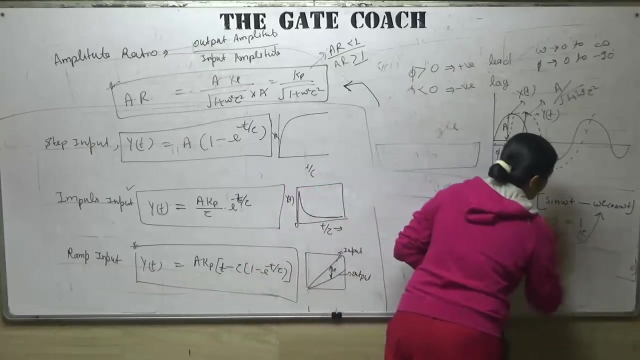 equations means partial fraction. you are talking about the partial fraction, I know. so in that case, if that was simply the inverse Laplace transform, I am giving you few questions today to solve for practice on the Laplace. or either you can do it or you can do it in a different way. 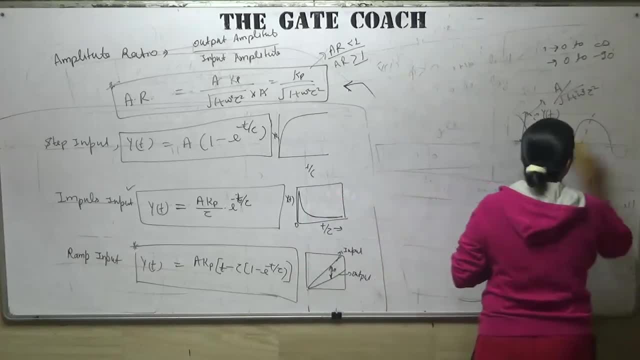 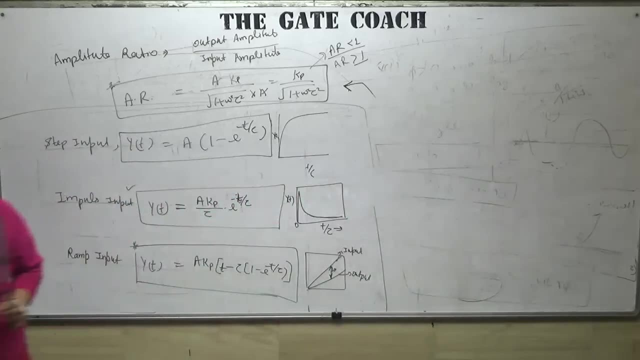 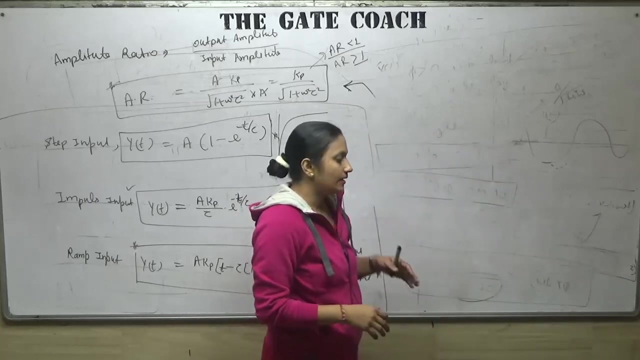 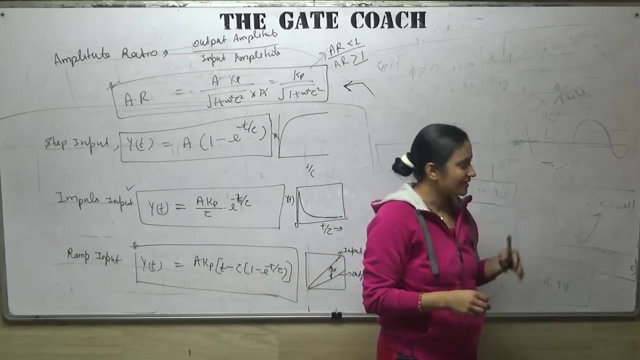 both and solve two, three questions given in your gate booklet provided by the coaching. solve few questions. for more and better understanding of the subject, I must suggest you just read whatever I have discussed, we have discussed today and just solve few questions from the booklets and from try to solve from last year gate questions. if you have any doubt, then ask. 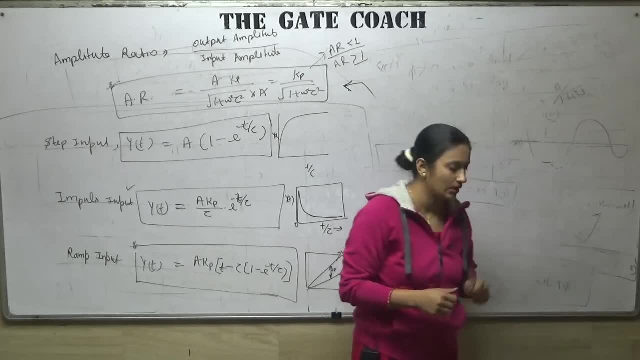 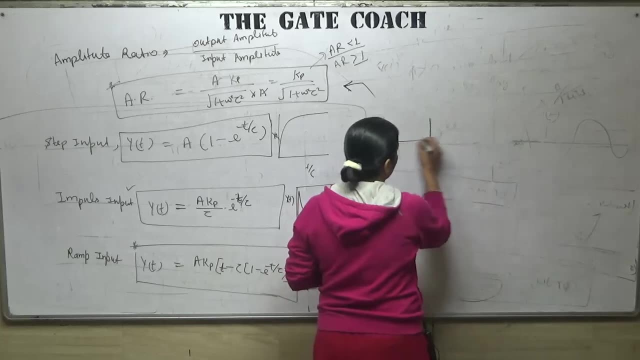 from this topic, from this topic that we have discussed tomorrow. I will explain you the applying the PSAception, the PSAads of partial fraction, that is, repeated and non-repeated equations. repeated equation, non-repeated equation is mean that is s plus 8 to the power Equaled.